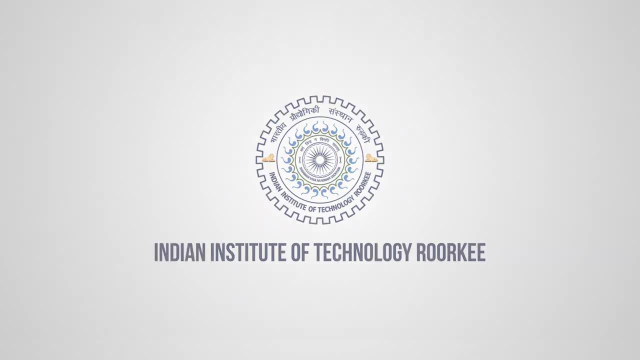 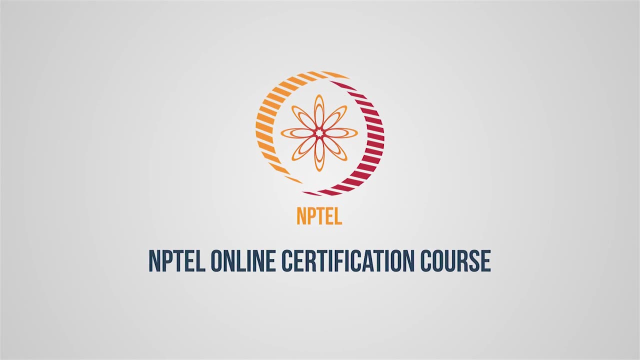 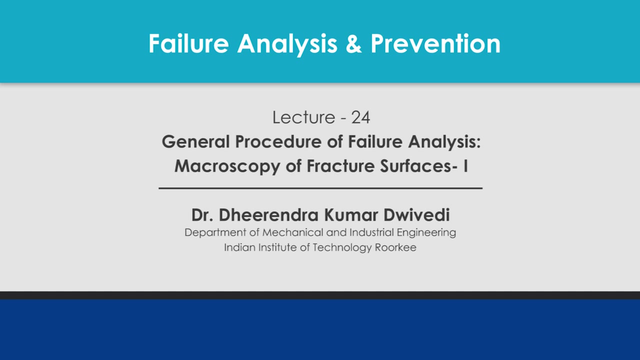 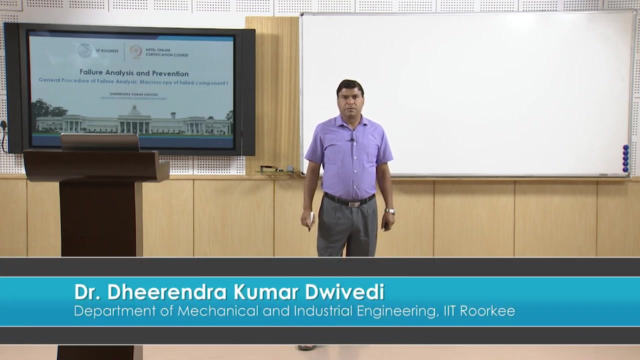 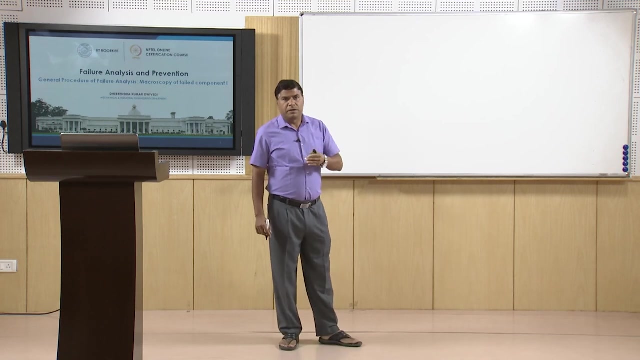 Hello, I welcome you all in this presentation related with the subject failure analysis and prevention. You know we have talked about the fundamental sources of the failure and in this presentation we will be talking about a specific aspect related with the general procedure of the failure analysis. Now, in this presentation, we will be talking about 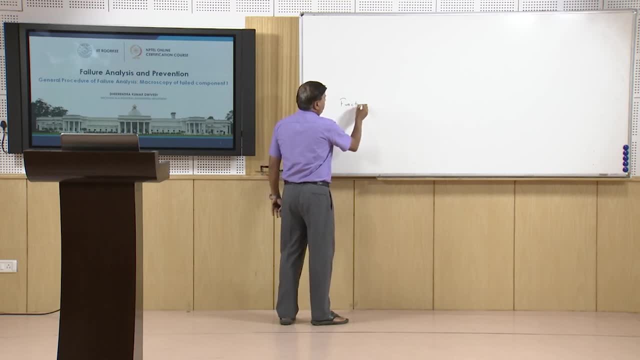 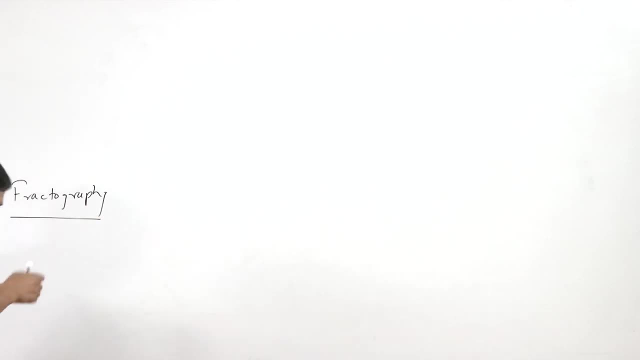 the like, say the fractography. We know that the failure of the component can occur in number of ways, like: if you have to define a failure means the component inoperable. This is the one way where it operates. another way, like component, operates but does not perform. 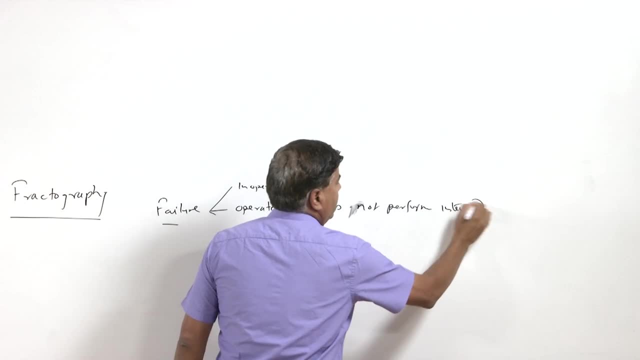 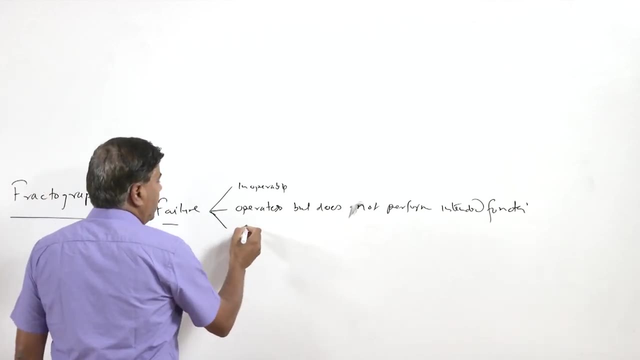 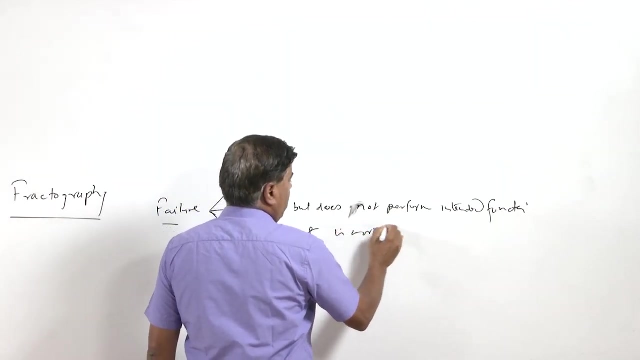 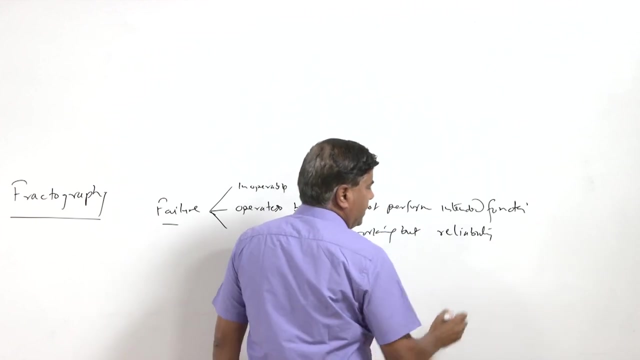 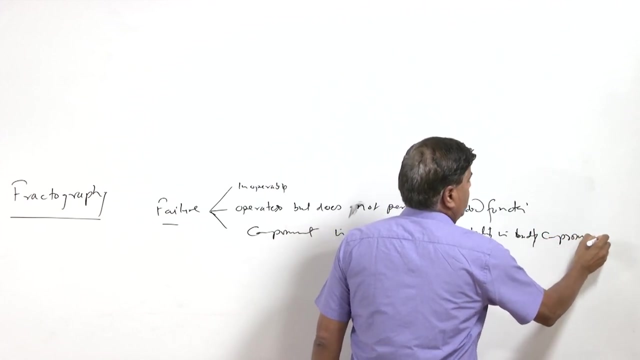 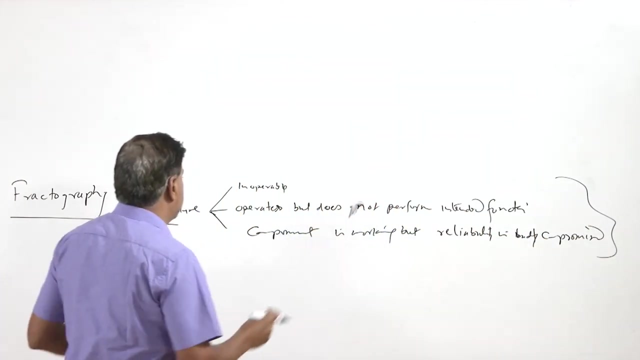 intended function. So again, in this condition we see that component has failed. and third one, where the component fails, I think the component is working, but reliability is badly compromised. So for this situation, for these are the three ways by which or three categories under which we say that the component 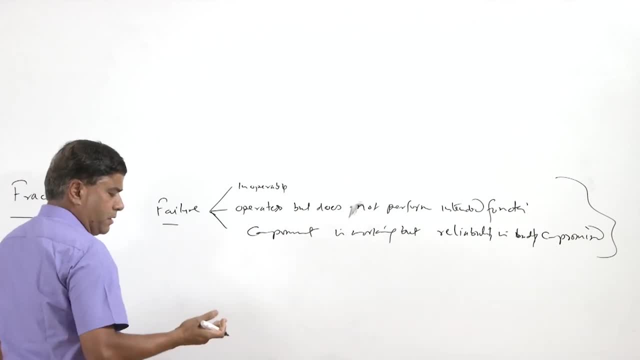 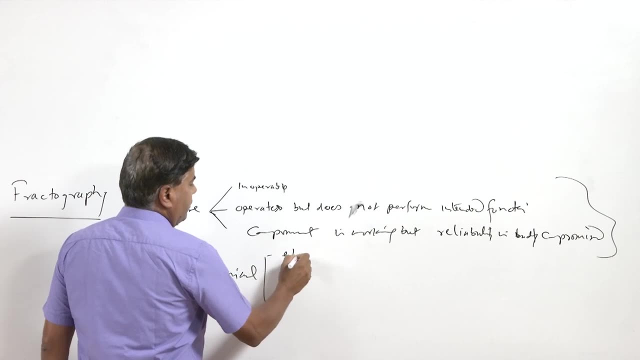 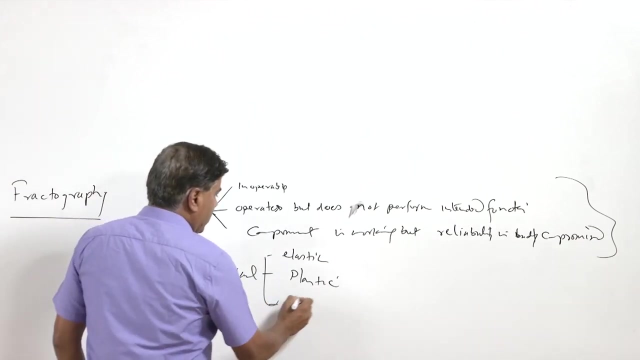 has failed for any kind of the component. But if it is about the mechanical component, then we say that when the elastic deformation beyond the limit, or when we say the plastic deformation beyond the limit, or when the fracture has taken place. So in case of the mechanical component, these are the three ways, or like say there is one. 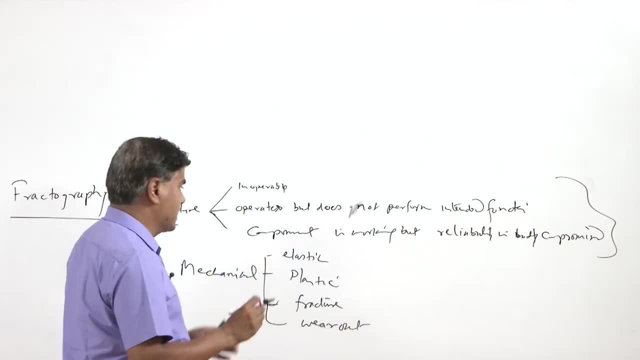 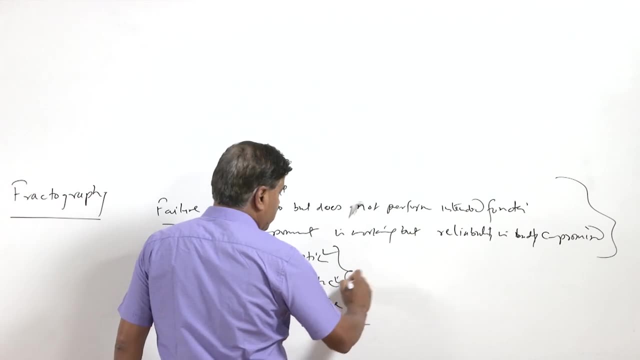 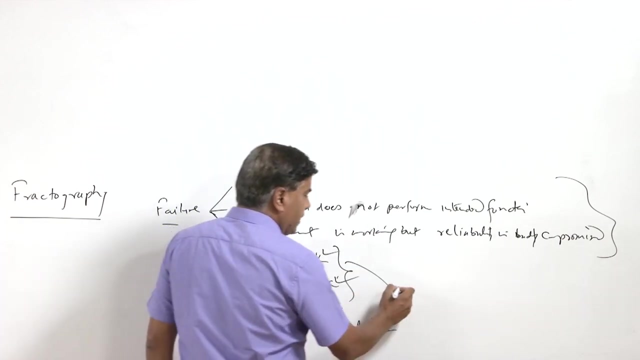 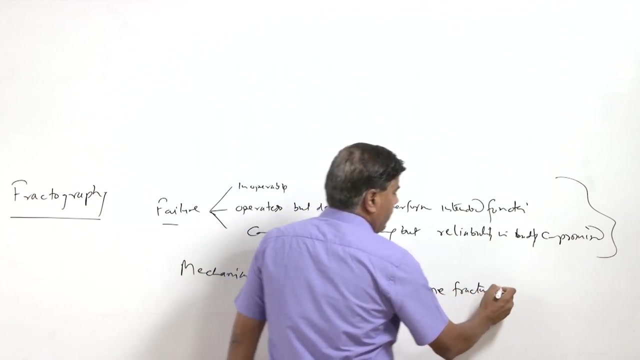 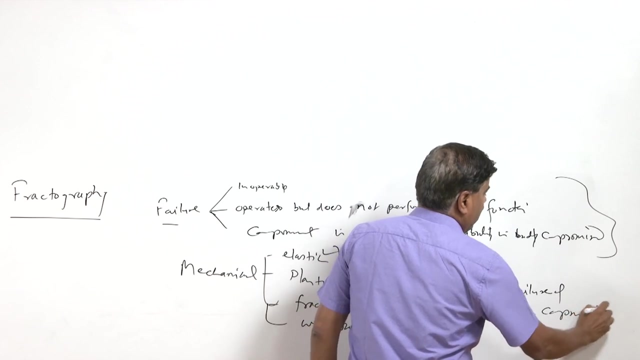 more wear out of the sample beyond the acceptable limits. So in these two cases, like elastic deformation beyond the limit or plastic deformation beyond the limit and the wearing out of the component, these are these three we can say as non fracture failures of mechanical component where elastic deformation or plastic deformation or wearing, 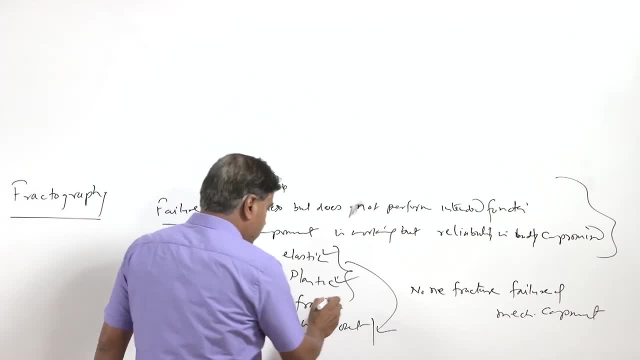 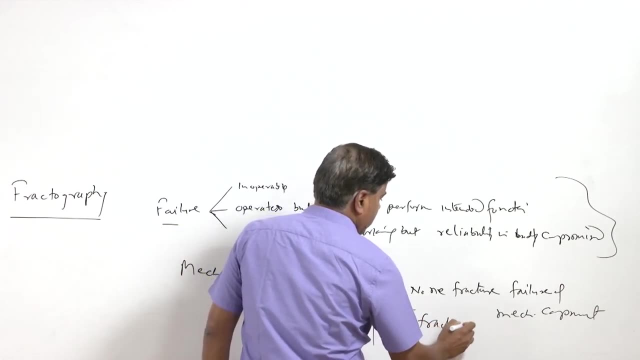 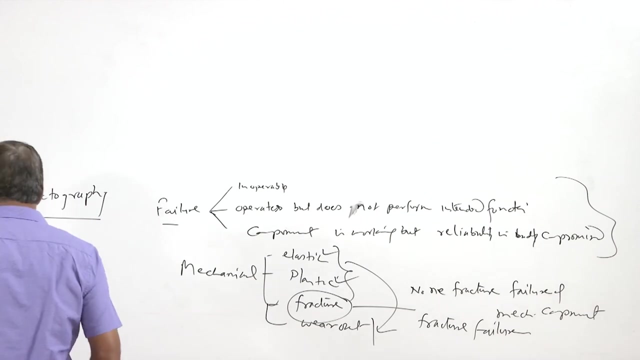 out of the component, So the component is beyond the acceptable limits. This is the one where fracture or suppression will be taking place. So this will be the like, the fracture failures, and others are non fracture failures, like elastic plastic deformation and the wearing of the component. 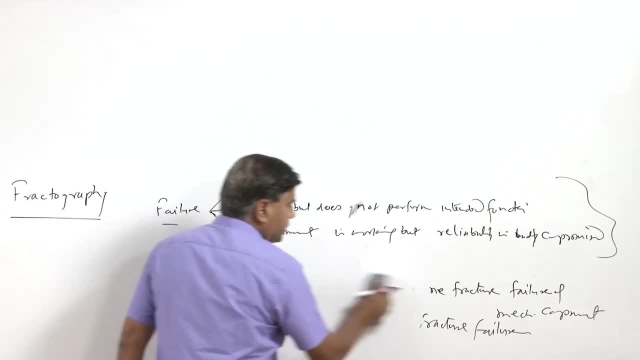 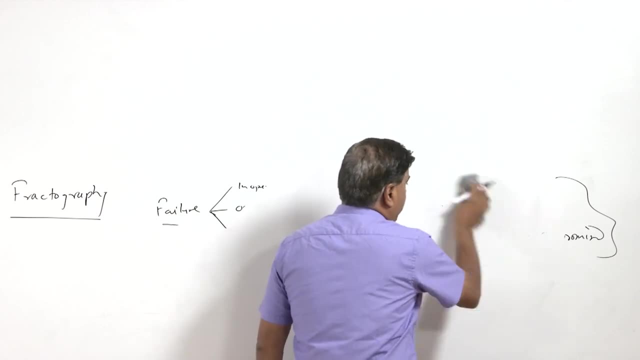 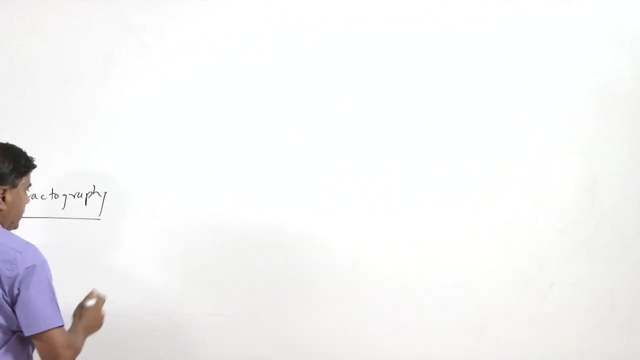 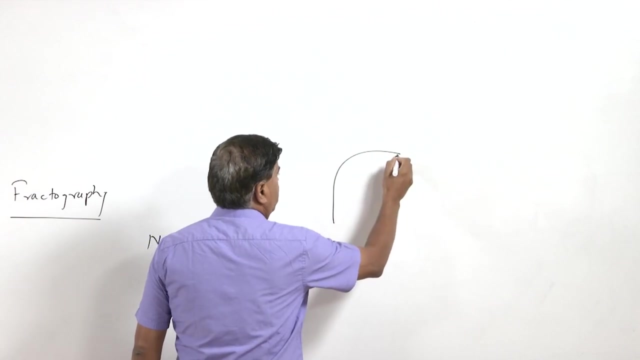 So to study the fracture related failures, our approach has to be different than the non fracture related failures of the mechanical component. So non fracture failures can occur in the number of ways like the component has been subjected due to the external excessive loading and it has got bent, so like it has been subjected. 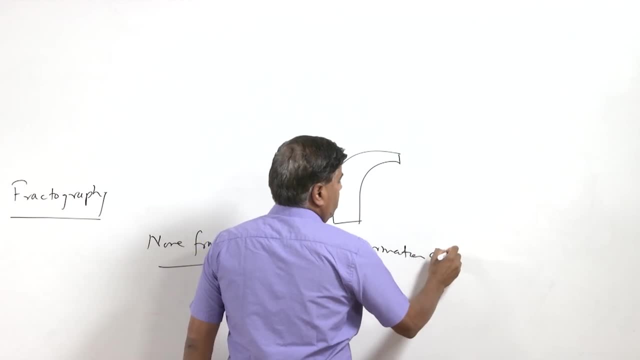 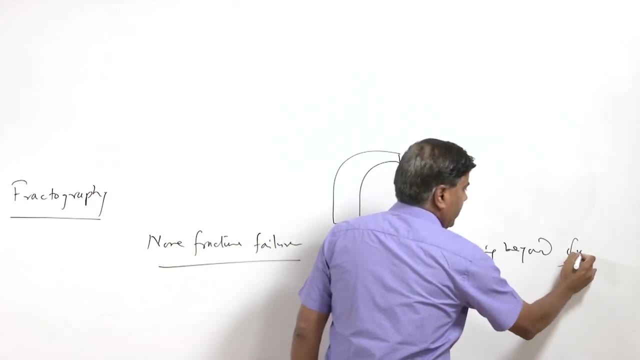 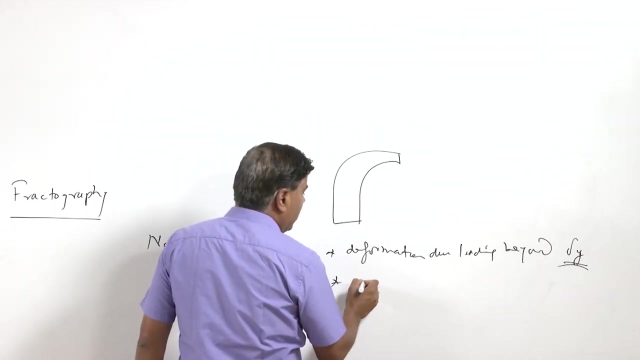 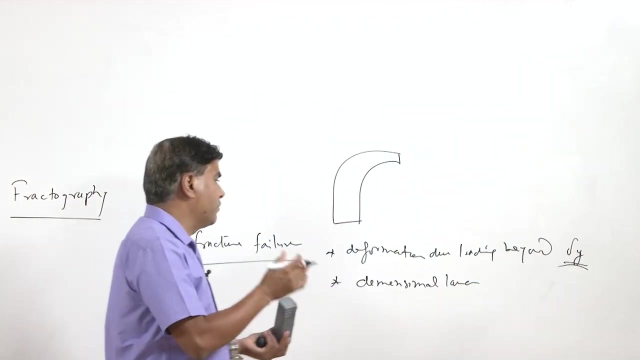 to the deformation due to the loading beyond yield strength of the material. So beyond the yield strength of the material. so this is one typical case or where, like the dimensional loss due to the variety of the dimensional losses has been excessive, due and because of which the component has started to not to perform as intended. 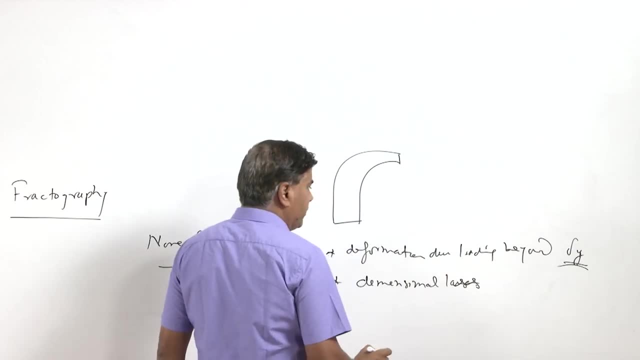 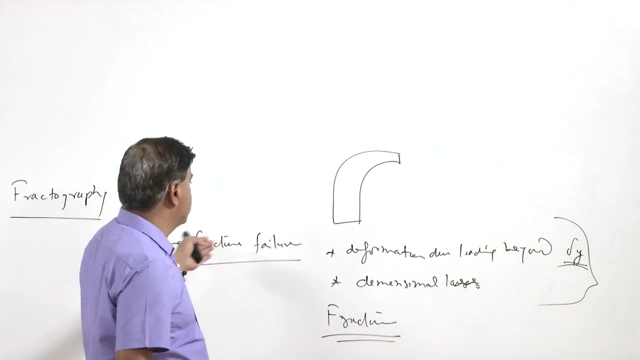 So these dimensional losses also will be leading to the failure and, if we see, sometimes the non-fracture failures eventually cause the fracture. So there may be possibility that initially the failure has started with the non-fracture failure. But if it continues for longer period then we will say that due to the excessive dimensional 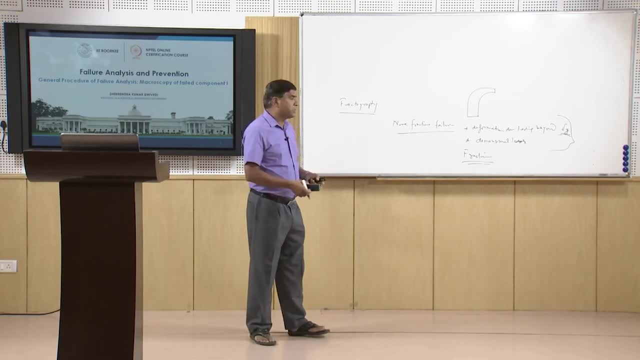 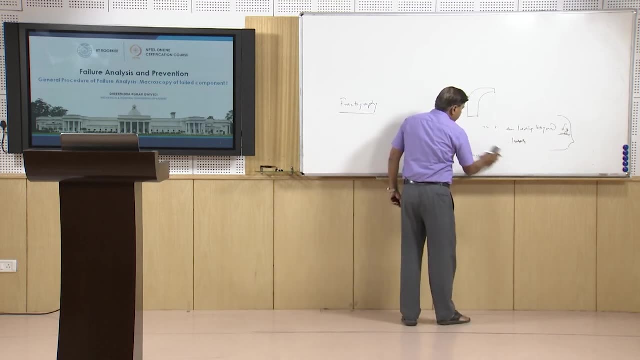 losses under the given set of the loading conditions, even the fracture may take place. So those but primary cause in those failures will be the different than those which will be occurring due to the fracture. Like the component will be defined even when it has started not to function, as per the 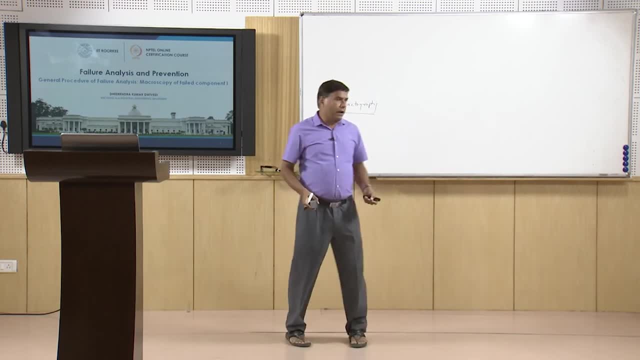 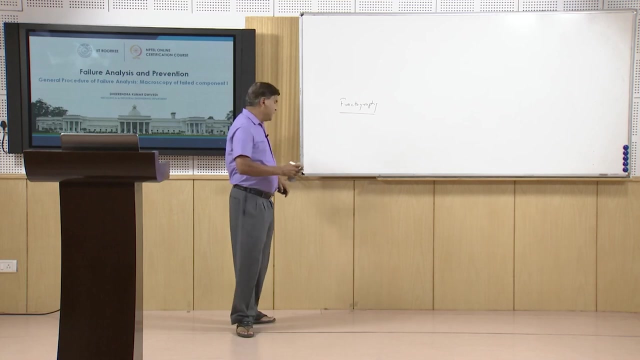 requirement much before than when fracture has occurred. So I mean to say, like the non-fracture failures eventually can lead to the fracture of the component. So like, if we see, like if any failure we have to group, then there can be those failures where the fracture occurs, or there can be the failures where no fracture occurs, or the 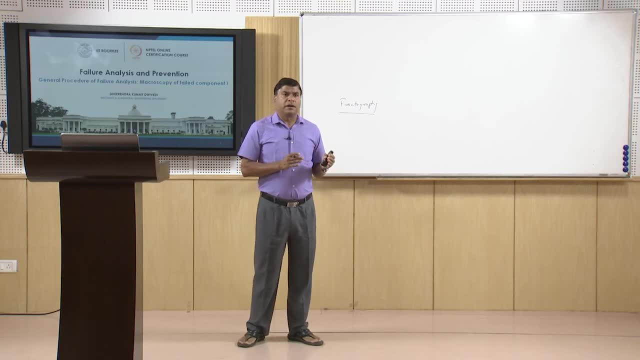 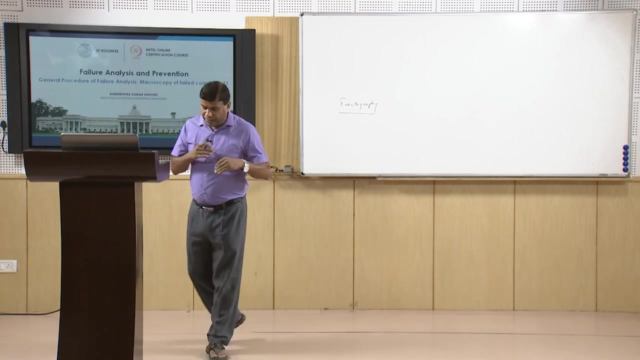 failure with fracture or without fracture, So without fracture failures. 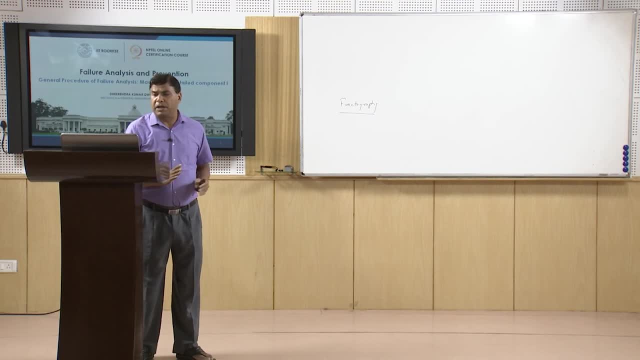 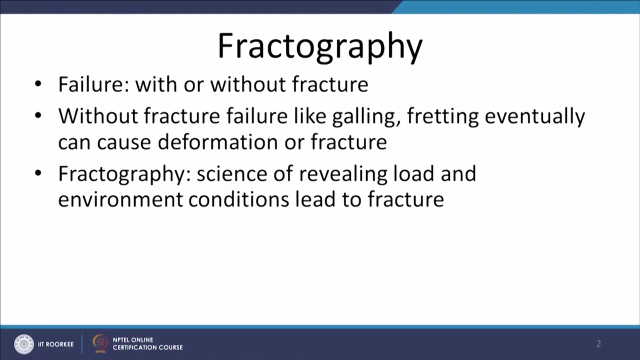 Then we have one special branch of the engineering or science wherein investigations are carried out primarily to see that under what loading conditions and under what environmental conditions failure has taken place. So, basically, the fractography is the science of revealing the load and environmental conditions. 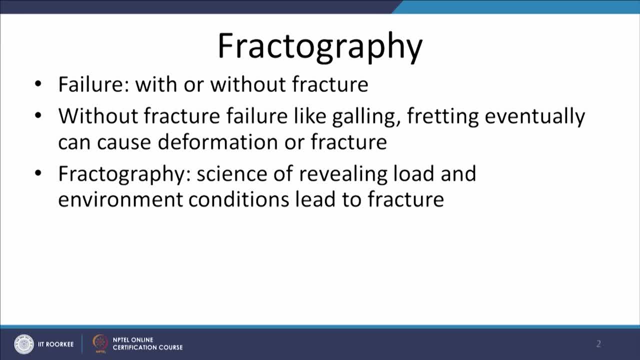 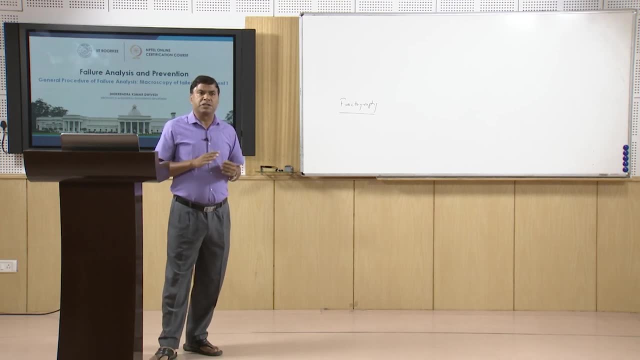 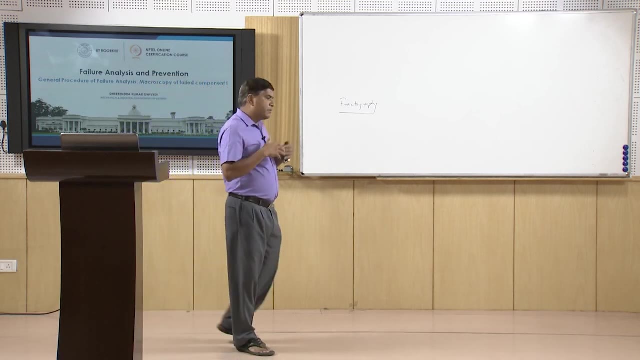 which have led to the failure of the fracture of the component. And what it uses? it uses the understanding of the different areas related with the mechanical failures and that is, and that is why we say that it uses three-dimensional interpretation of the appearance of the broken part wherein, like we will be trying to observe the fractured 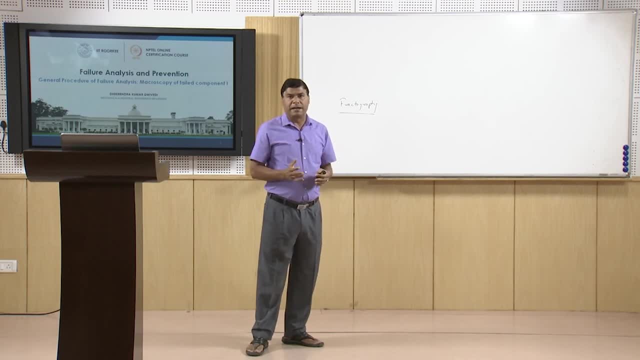 component or broken part visually using the naked eye. then we will be using the macroscopy and then we will be using the mechanical part. So this is the macroscopy of the failed part, wherein the low magnification cameras, low magnification lenses, stereoscopic cameras and even the scanning electron microscopy. 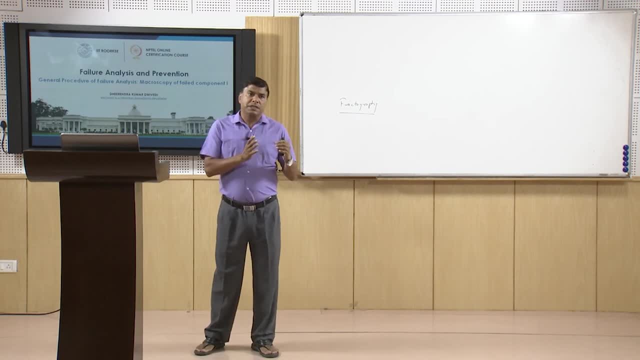 is used at a low magnification. So these are the macroscopic observation of the failed part and then further we carry out the microscopic observation of the fracture part. So the combination of the various approaches help us to understand and to understand the failure of the fractured component. 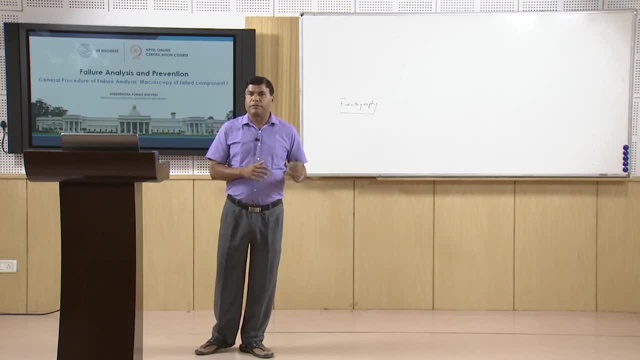 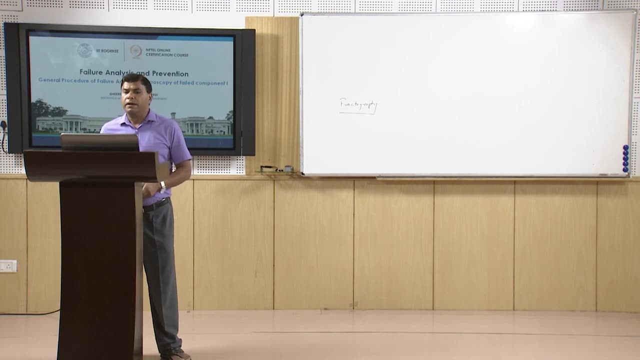 So this is the way to reveal the loading and environmental conditions under which failure or the fracture of the component has taken place. So that is why what we say, that it uses three-dimensional interpretation of the appearance of the broken parts. So when the fractography is carried out, it helps in identifying the loading events. 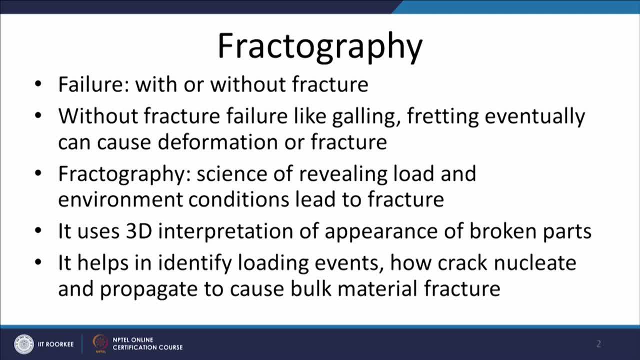 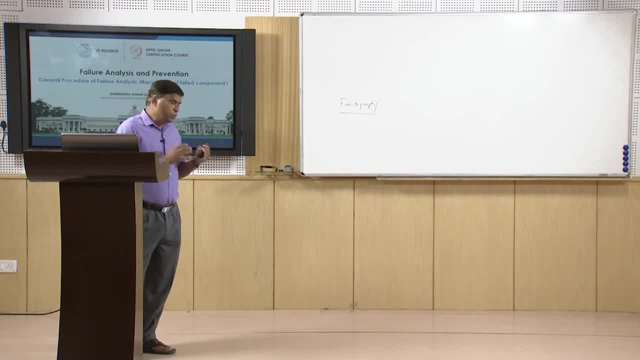 how the crack has nucleated and it has propagated during the fracture of the broken part. So that is why we say that it uses three-dimensional interpretation of the appearance of the broken parts. So when the fractography tool is systematically applied, it will help us to know the kind. 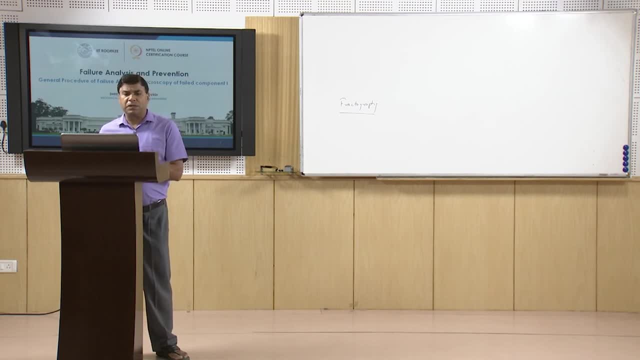 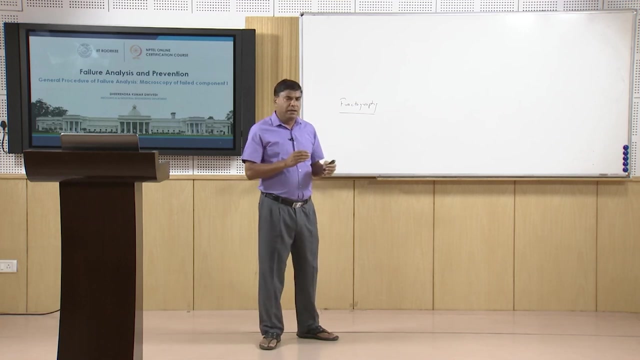 of loading conditions, the where crack has nucleated and how it has propagated during the fracture of the bulk materials. So what we need to do for the fractography of the broken parts, they are basically, as I have said, There is a macroscopic observation and the microscopic observation. 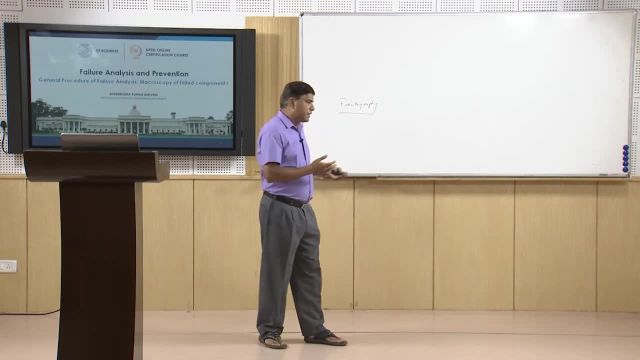 So for macroscopic observation, first of all, we start with the observation of the failed component using the naked eye, where which we can say as the observation starts with the visual examination of the failed component, starting from very low magnification, like using naked eye, then low magnification lenses, then stereoscopic microscope, and then 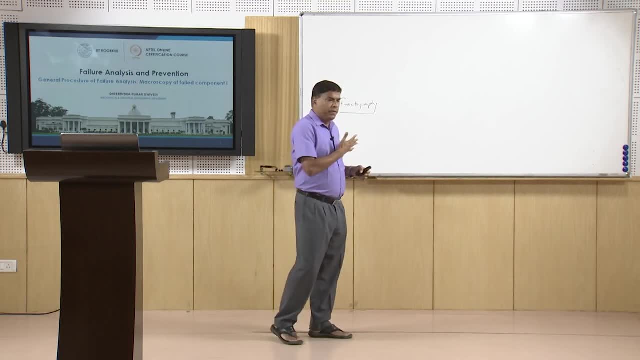 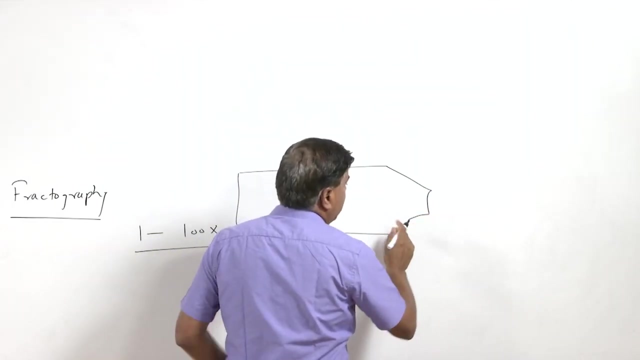 scanning electron, So these are normally done at a very low magnification, which may be in the range of 1 to 100 X, and when these observations are carried out, it reveals lot of information, like if the failed component is really very big and if it has failed like this and is 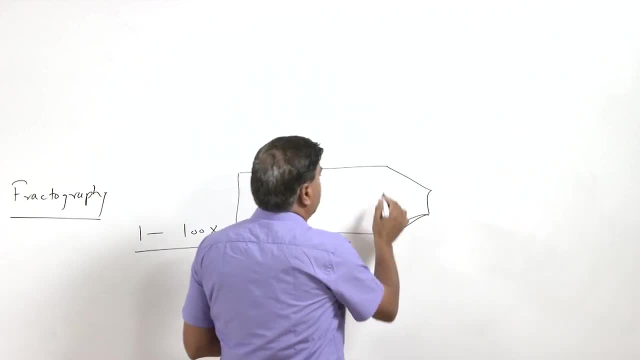 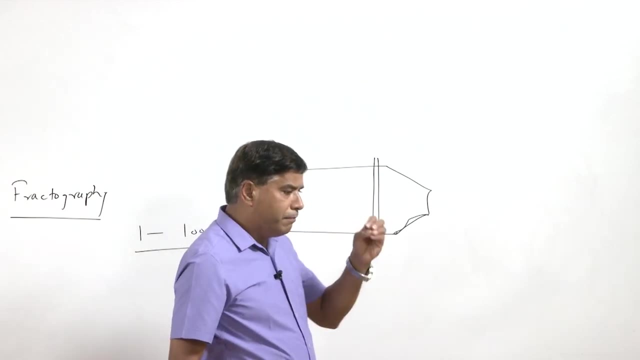 showing in this manner what it will be. showing that cross section actually of the component this component has reduced significantly means no microscope or a scaling electron microscope can show such kind of the variation in the failed component. variation in cross section or the deformation in the component or the wearing of the component cannot be. 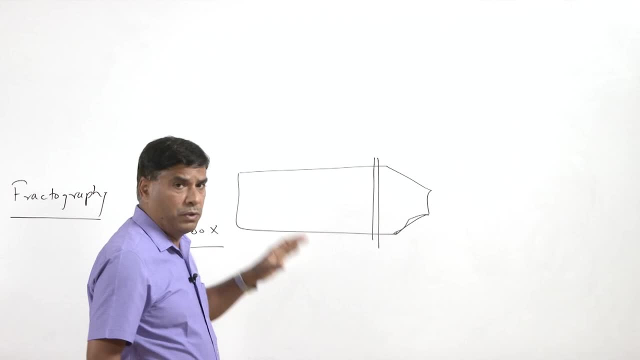 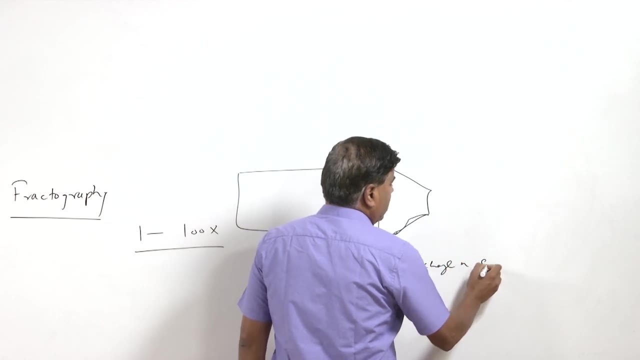 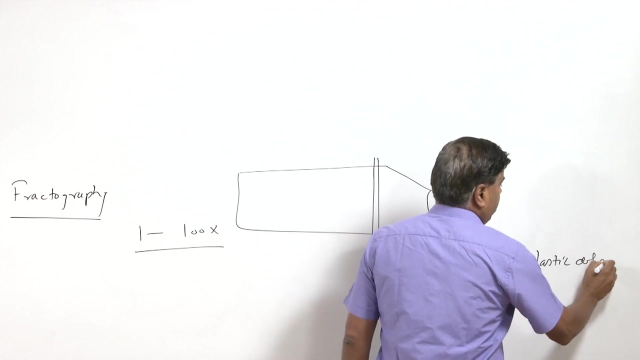 observed. It can simply be observed through the visual examination. so the major change in cross-section of the component can simply be observed through the visual examination and this will indicate that really component has been subjected to lot of plastic deformation prior to the fracture and which indicates that really this is the. this is where the material has been subjected. 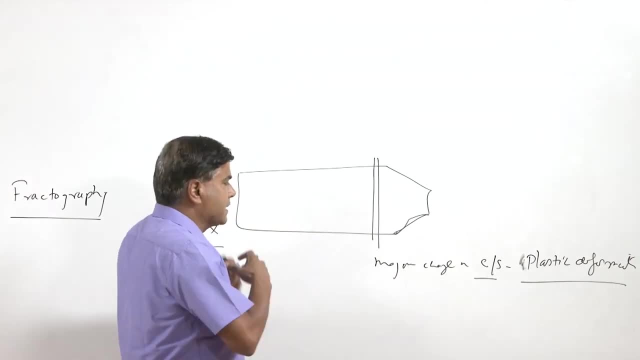 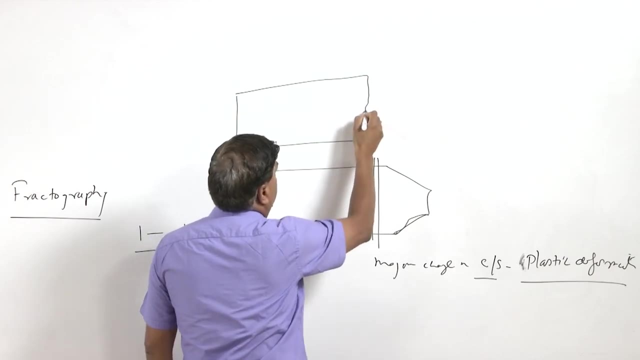 to the deformation. material is ductile and it has been. it has given enough indication prior to the fracture. there can be another possibility when the same section, component may feel abruptly Without in giving any kind of indication. so in this case there would not be any change. 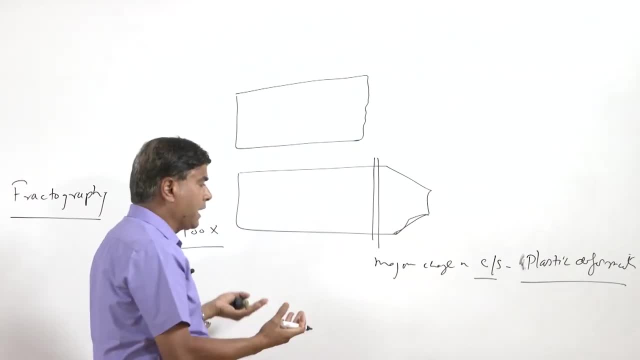 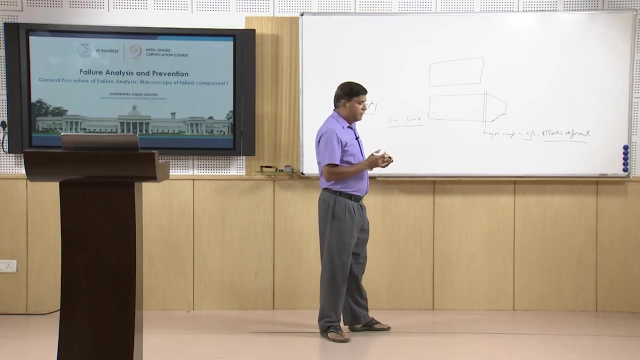 in cross-section of the component. So such major changes can only be observed through the visual examination of the broken component, and these will indicate lot of information. these will reveal lot of information about the stress system under which component has worked, the kind of the load which has been. 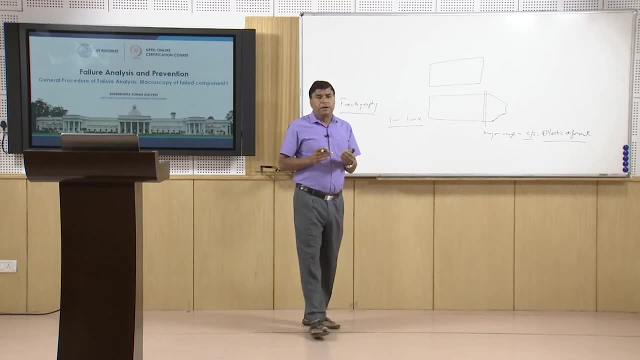 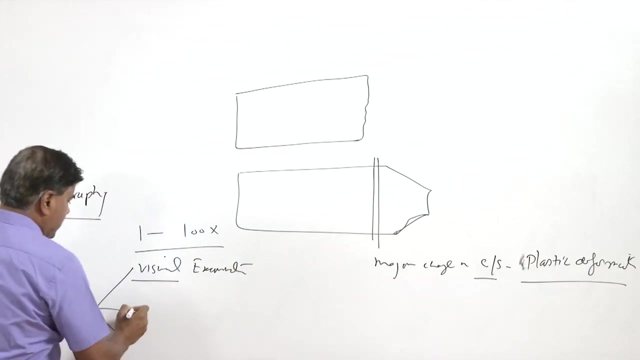 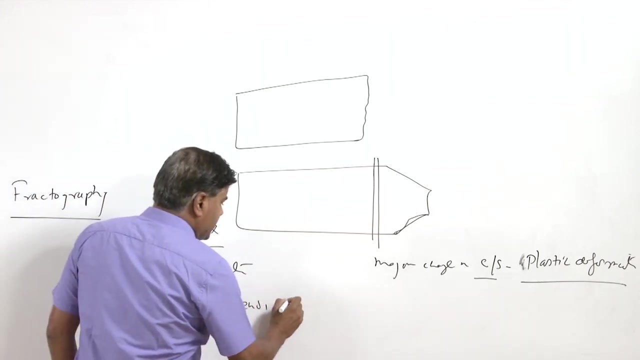 experienced by the component. So, for doing the fracture, For doing the fractuography, there are systematic approaches. primarily, it is like say we can put it in three categories: visual examination is one. the macroscopy, which uses the lenses, or stereoscopic microscope, or scanning electron microscope. 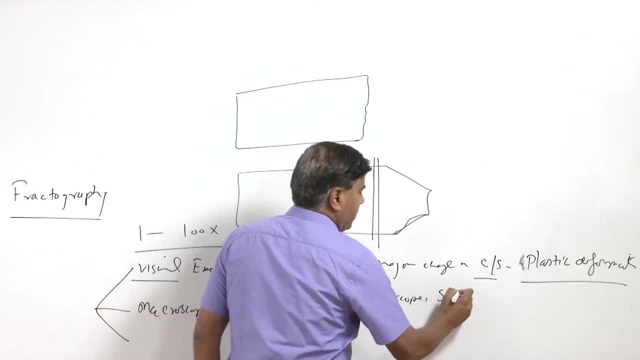 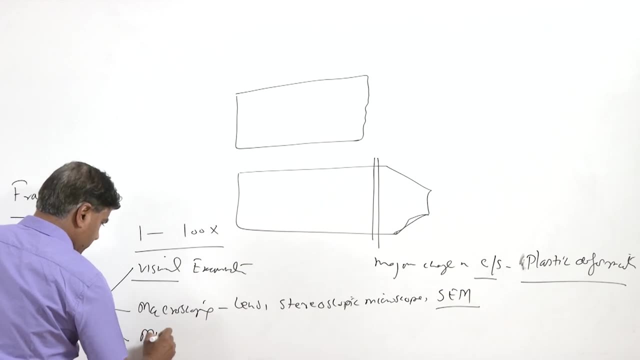 So these are the three categories, So the macroscopy, So the macroscopy, So all these are used at low magnification like 1 to 100. Then the third aspect related with the fractography is the microscopic observation, microscopy. 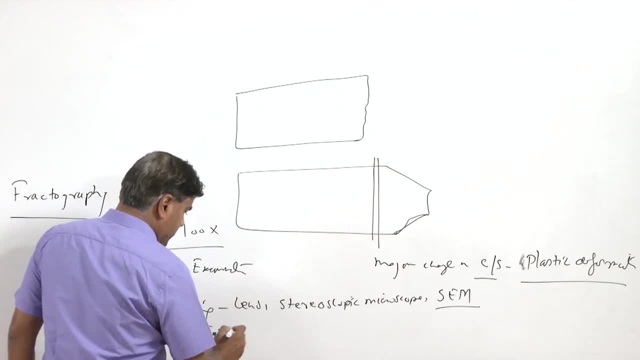 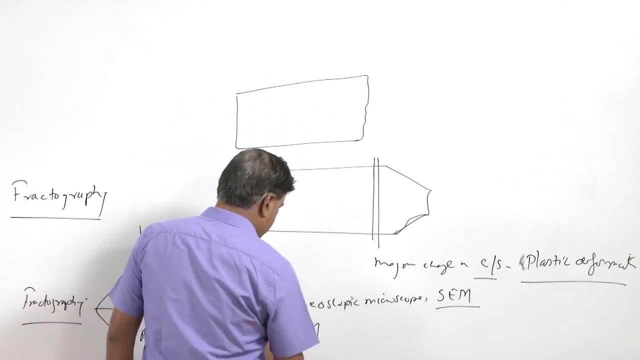 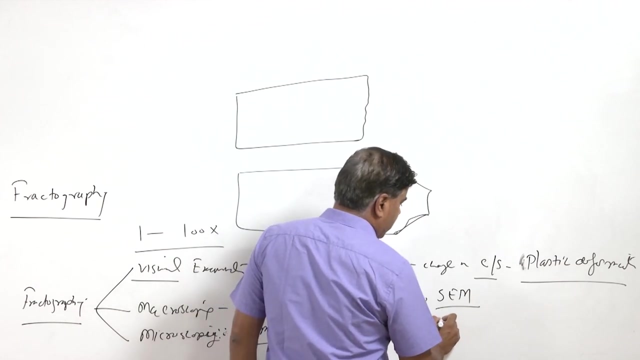 which we can say microscopy of the fracture surface. so it is carried out normally using the scanning electron microscope or transmission electron microscope And this can be done over a very wide range of the magnification, from like, say, 100 to even like 1 lakh magnification range. 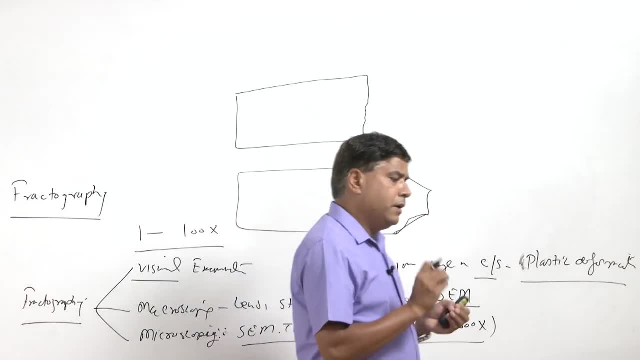 So this is very wide range. it allows us to look very closely in various microscopic features which are generated in course of the fracture of the bulk materials and they will be indicating, they will be giving us a very wide range of magnification. So this can be done over a very wide range of magnification, from, like, say, 100 to even. 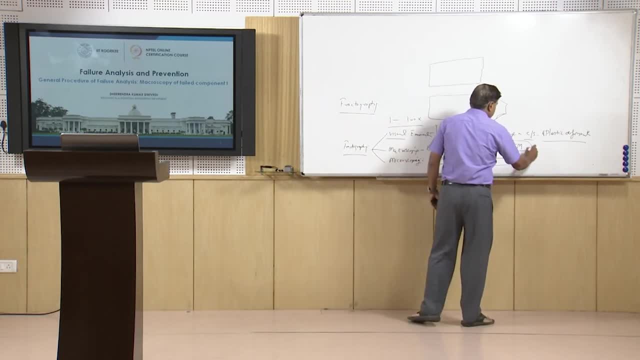 like 1 lakh magnification. So this is very wide range. it allows us to look very closely in various microscopic features which are generated in course of the fracture of the bulk material. and it is very wide range. so while they are communicating, they will be giving idea about the kind of 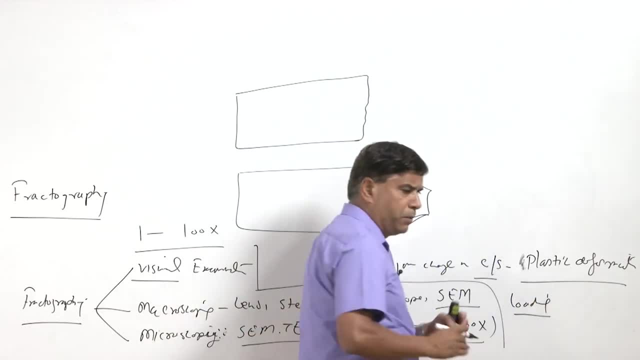 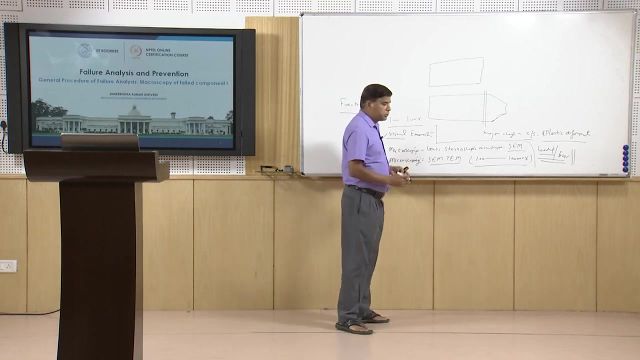 the loading conditions or the type of load, the- whether load was monotonic or it was cyclic, or the kind of environmental conditions under which failure has taken place. So, loading and the environment under which the failure has taken place, these things can be investigated through the fractography using these three approaches, all these three techniques. 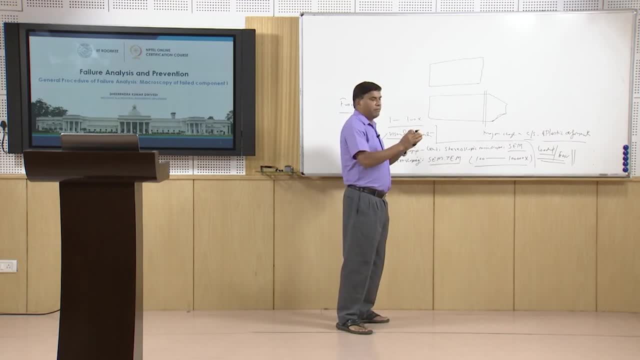 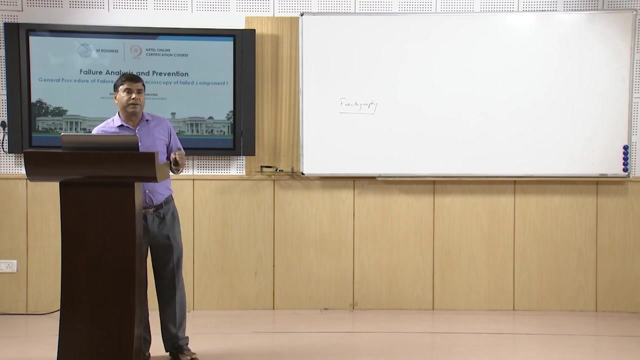 should be coherent with regard to the mode of failure, fracture or the mechanisms which will be leading to the failure of the or fracture of the component. Now what for it is carried out actually like spectrography, as I have said, it helps to identify the loading conditions and the environmental conditions which have led to the failure of. 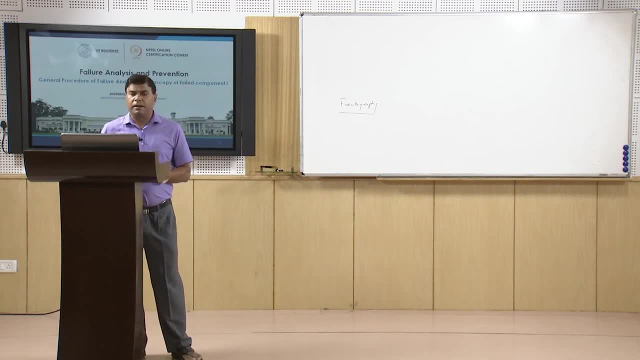 the component and, in line of that, the basic purpose of the spectrography is that it helps to determine the root cause of the failure among, the. so root cause of the failure will be among the fundamental sources of the failure, like, if, the, if some of the fundamental sources. 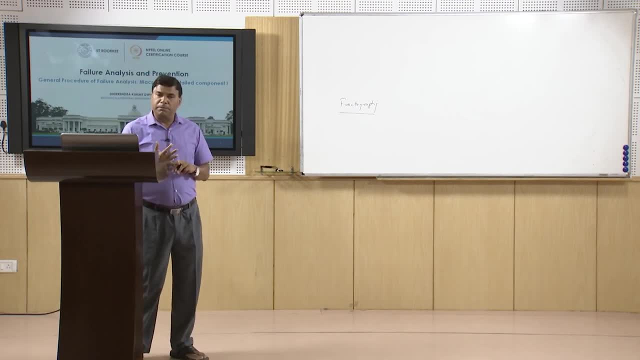 of the failure, like improper, deficient, improper or deficient design, improper material selection or improper manufacturing, improper service conditions, improper maintenance, improper assembly And, you know, Improper maintenance plan. so all these things, if they have been improper, then they will be leading to the conditions, with regard to the load and environment, such that the fracture. 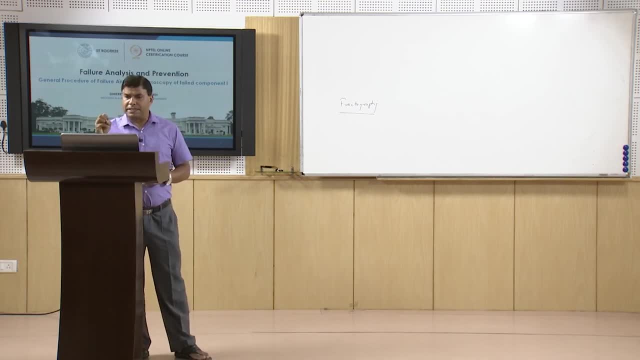 will be occurring. So those things are established among the fundamental sources of the failure which one was basically responsible for. fracture of the component. So that is what is identified through the spectrography. so determination of the root cause of the failure among the fundamental sources of the failure. 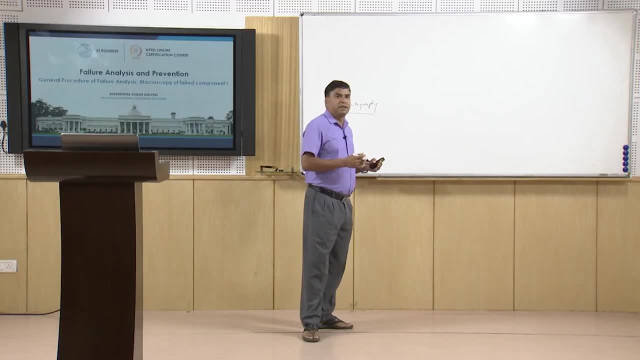 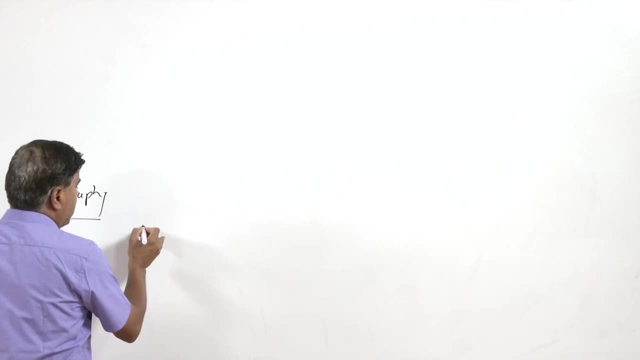 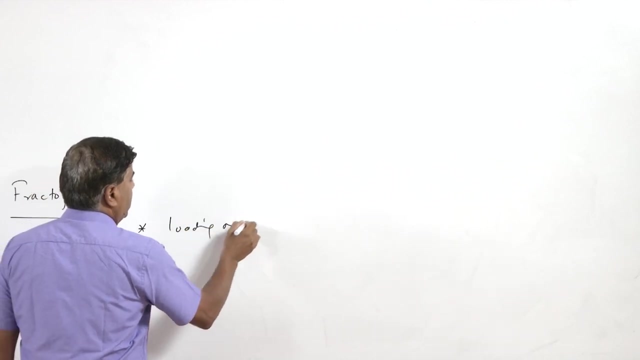 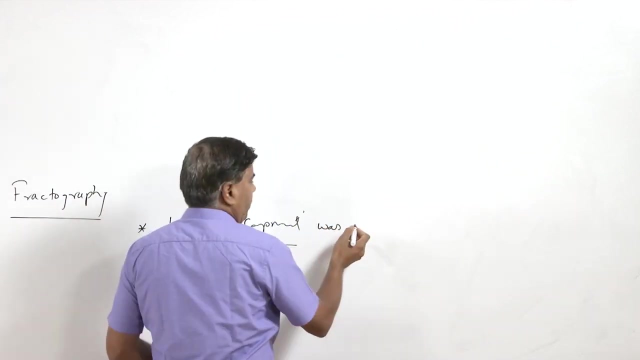 So, apart from that, how the spectrography helps in determining the root cause of the fracture. So whenever there is spectrography is carried out, it helps in determining whether the loading on the component, loading on the component which has fractured, was So it is. 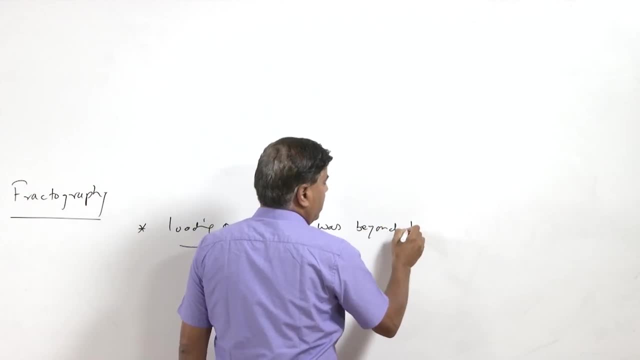 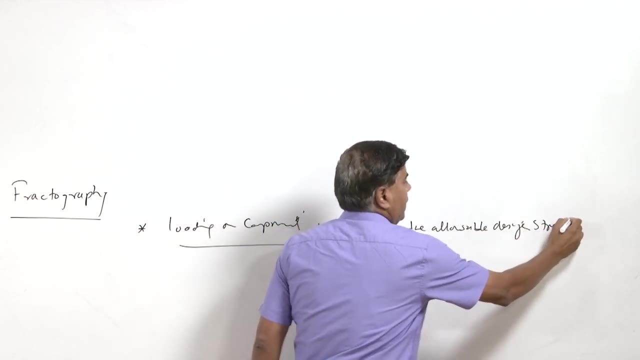 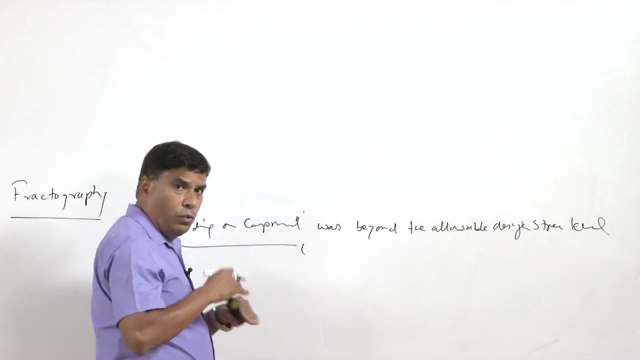 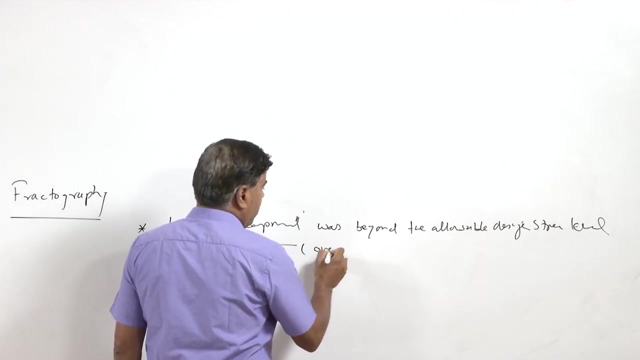 So it is. So it is beyond the allowable design stress level. so this is one thing. that so it means whether the component was overloaded or not, and because of which fracture has occurred. So if the failure is due to the overloading, that is what is identified, basically. so, during 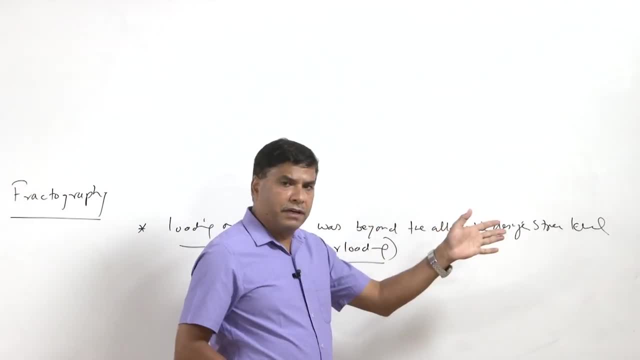 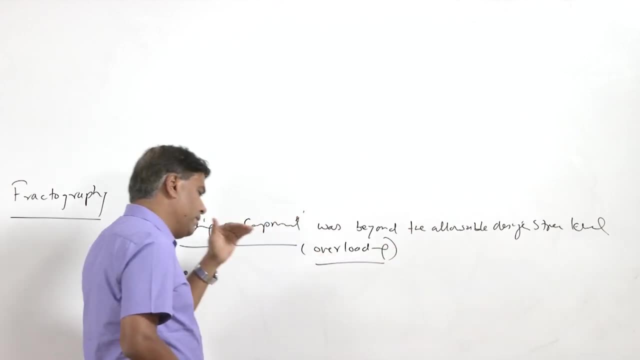 the service. if the component was overloaded, it will show the different kind of feature as compared to the case when the failure fracture has occurred below the within the allowable or the design stress level. So if the applied stresses are more than the allowable, design allowable or the design 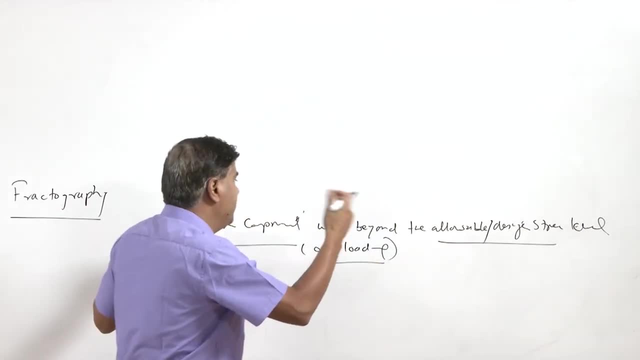 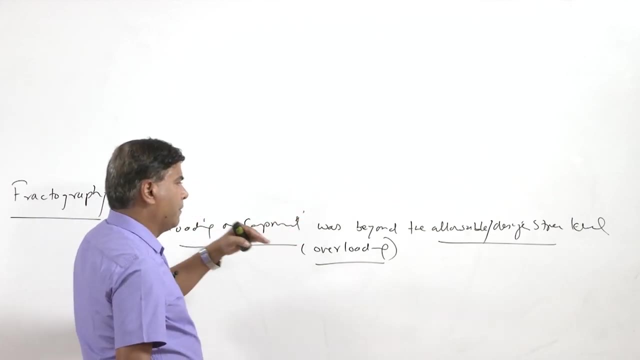 stress levels, then the surface features will be different than the case when the component is. fracture of the component is occurring under the stress levels which are well within the design stress levels. So this is one thing. it helps to rule out the possibility of the overloading or it will. 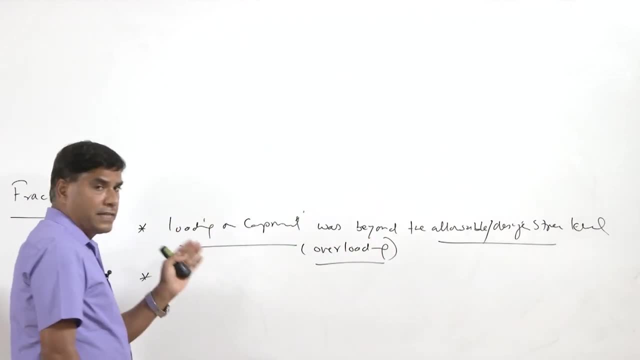 confirm the possibility of the overloading for as a cause of the fracture. The second one is that, whether the failed component, component material or the material of the component Had the required properties or not, as expected by the design engineer, so it will confirm. 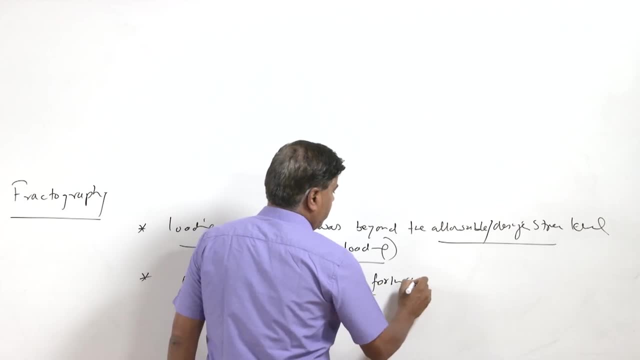 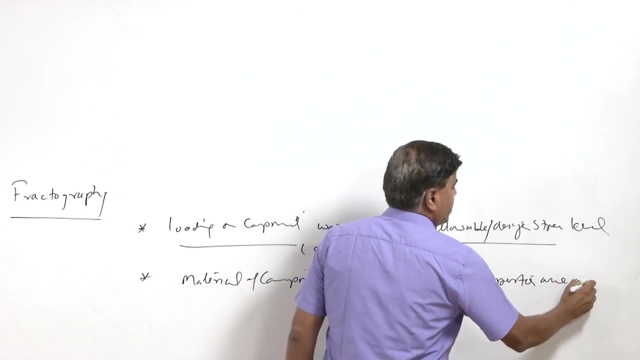 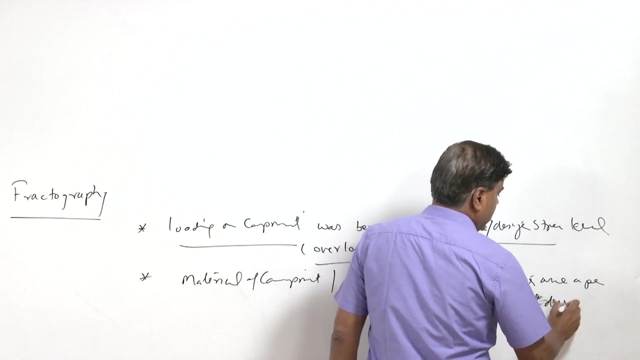 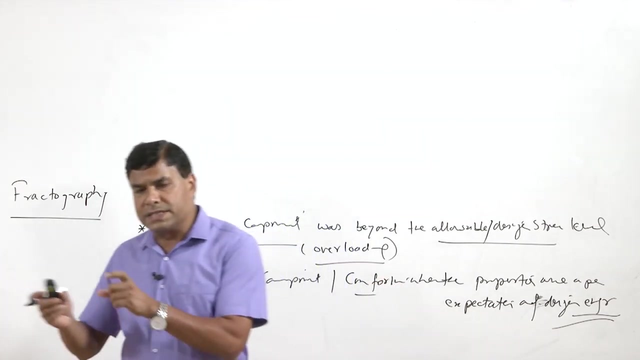 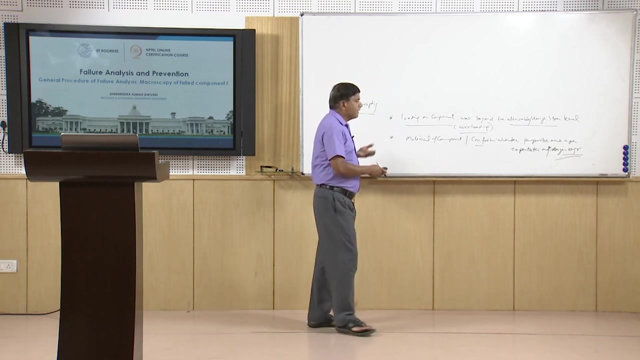 basically, it will confirm whether the properties were as per expectation, as expectation of the design engineer or not. Like the design, engineers, will assume that the material will have these set of the properties if due to some kind of the fault with the material. if the material does not have those, 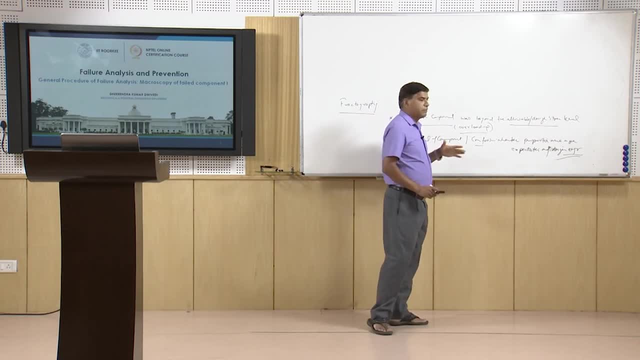 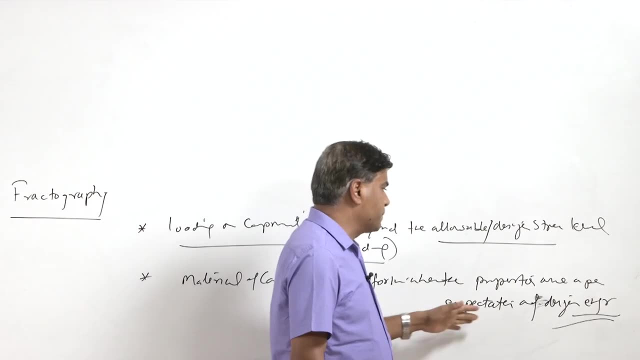 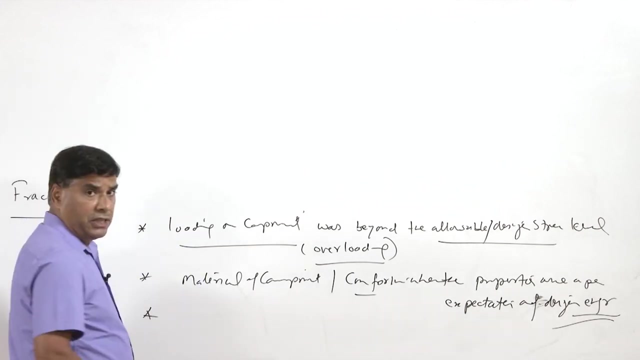 set of the properties, so it will be leading to the failure of the component. So that kind of confirmation if the material is having the required set of the properties or not, as expected by the engineer, that is what can be Conformed to the fractal graph. and the third one is that if there are discontinuities in 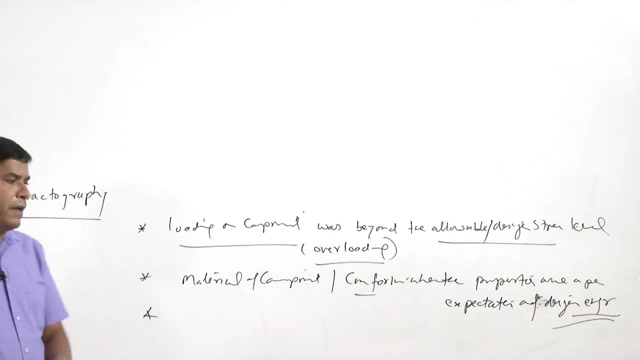 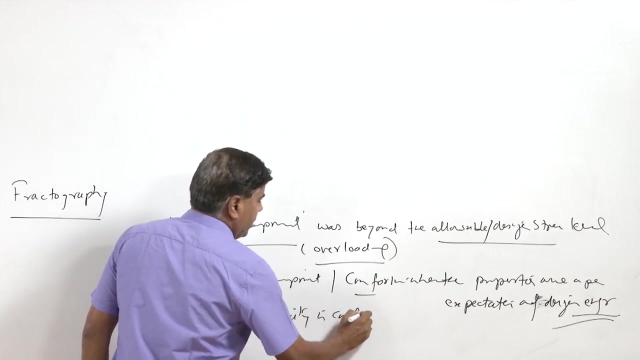 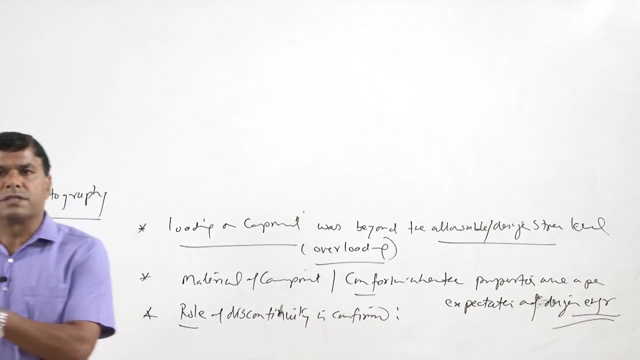 the materials. so if they have contributed towards the fracture, So the role of the discontinuity is confirmed with regard to the fracture. So whether really Maybe the discontinuities have played a crucial role towards the fracture or not, that is what 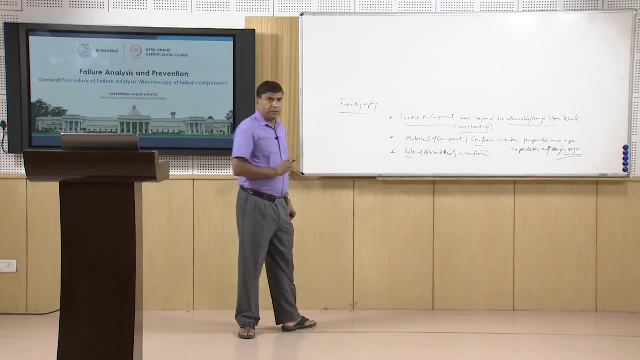 can also be identified through the fractography. So whenever fractography is carried out, it helps in ruling out the possibilities. these three possibilities: One: if the material has been subjected to the overloading, if the material had the desired set of the properties, as expected by the design engineer, or if the discontinuity is present. 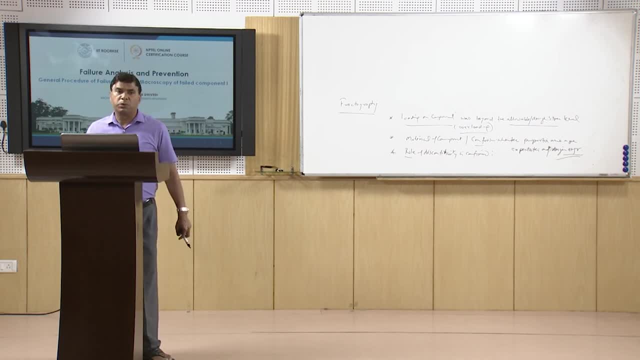 in the failed component had played a crucial role or not towards the failure. so that is what also can be identified Now, like if the fracture has taken place. so how to group or categorize these fracture? So, based on the appearance means, on the macroscopic observation, the fractures are grouped in four. 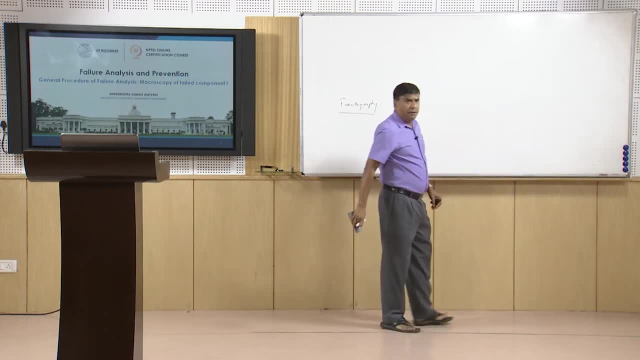 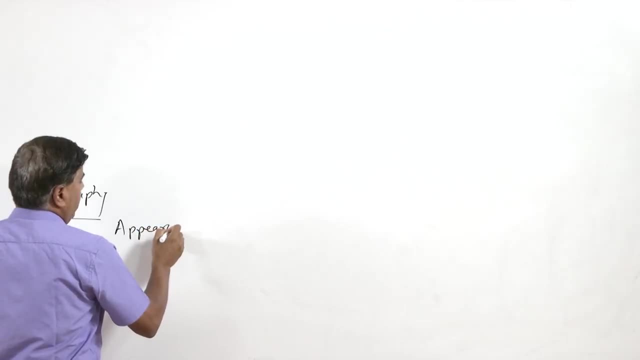 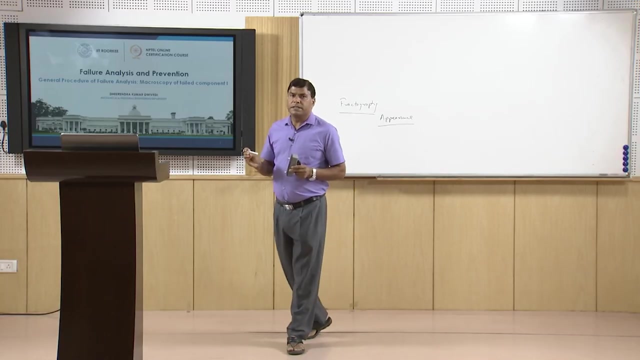 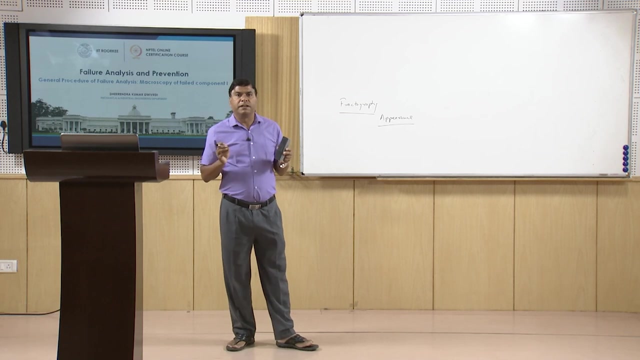 or five. There are, like, say, the five types of the fractures based on the appearance of the failed component, and this include, like the ductile fracture, where significant plastic deformation of the failed component will be taking place. the brittle fracture, where no indication of the deformation will be there prior to the fracture. the fatigue fracture, where the fracture is. 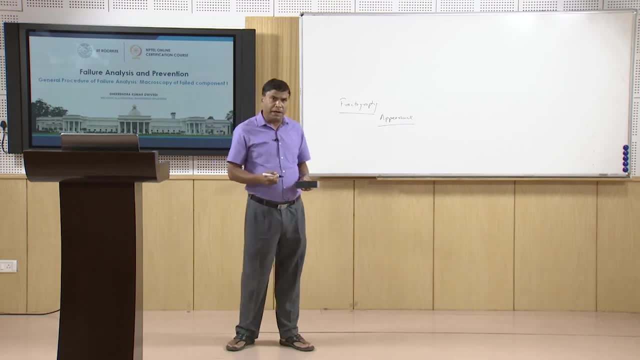 the fracture surface will show the typical appearance of the beach marks indicating that the component has been subjected to the fatigue loading. So the fatigue fracture will be unique and the different with regard to the ductile and brittle fractures. in terms of the fracture appearance, because it shows the typical beach. 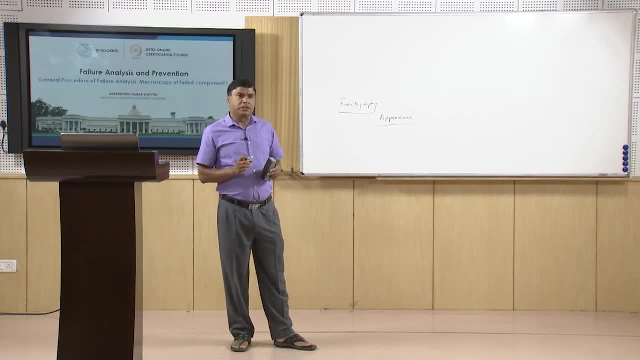 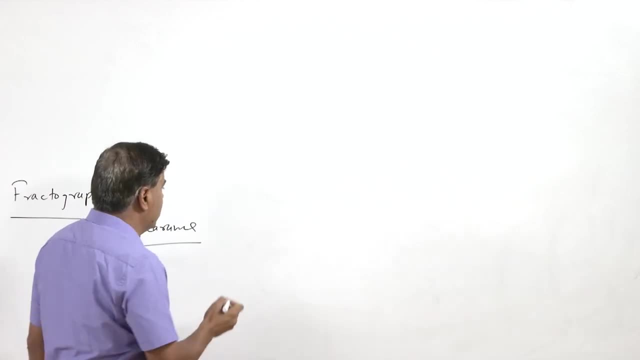 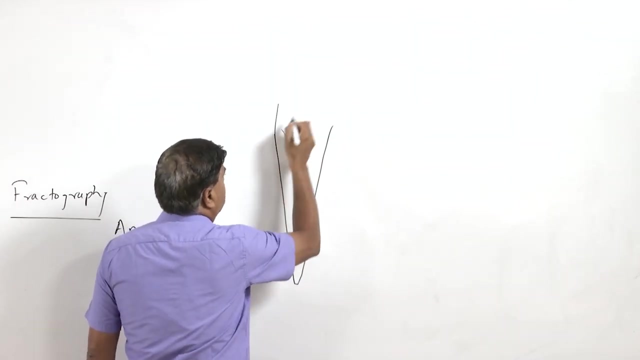 marks on the fracture surface. The creep fractures show again the different kind of behaviour where, because the creep will be occurring at high temperature, where the material may show lot of the ductility, So this is one where the reduction in cross section has been up to such an extent that 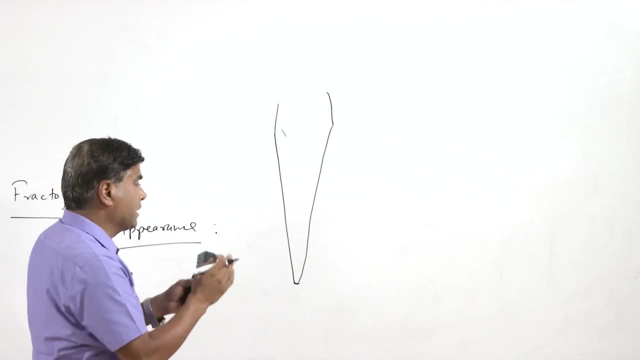 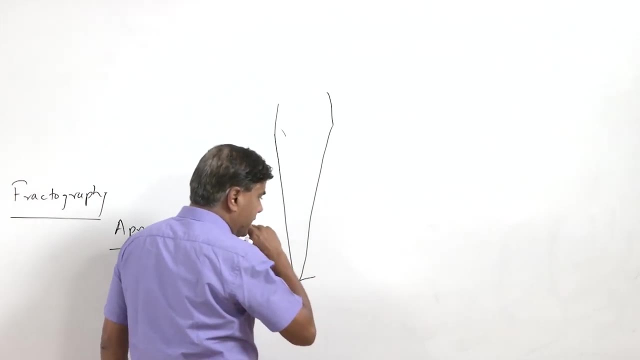 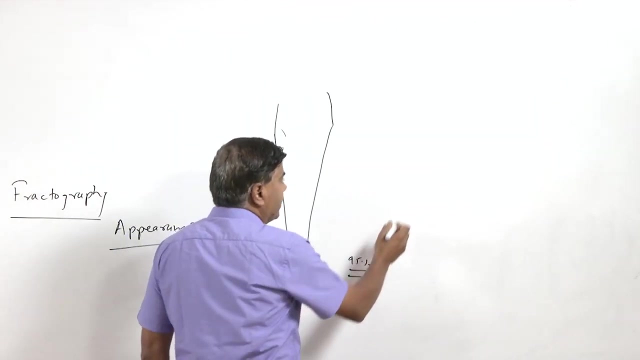 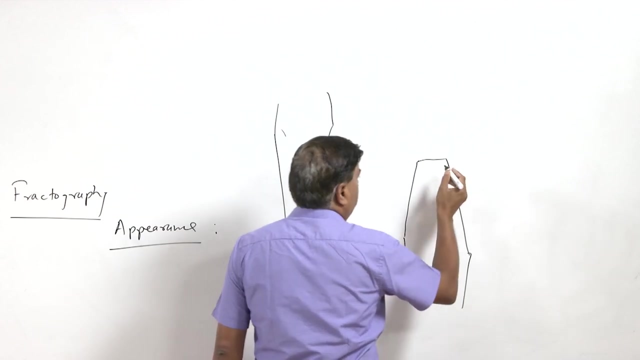 a component has been subjected to do a component, cross section has been reduced to such an extent that it is like the percentage reduction is like, say, more than 95 percent. So this is one possibility, Another one where what we will say that although reduction in cross section is not much, but 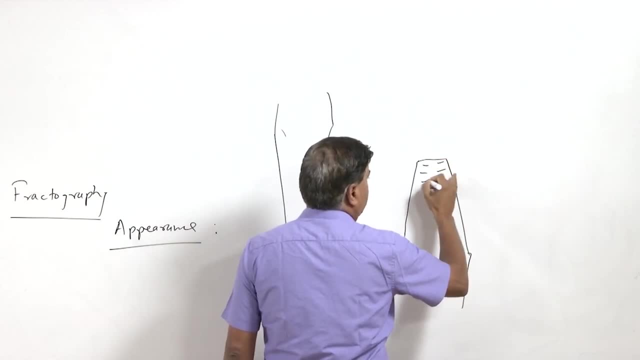 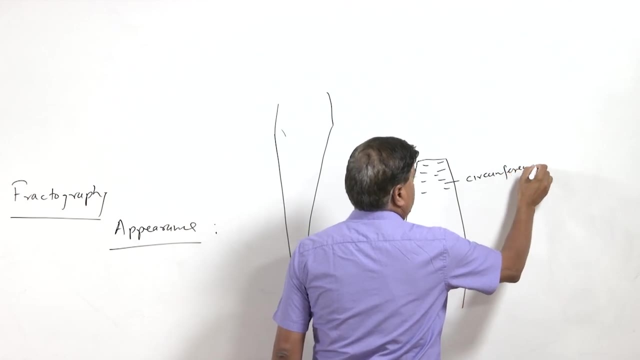 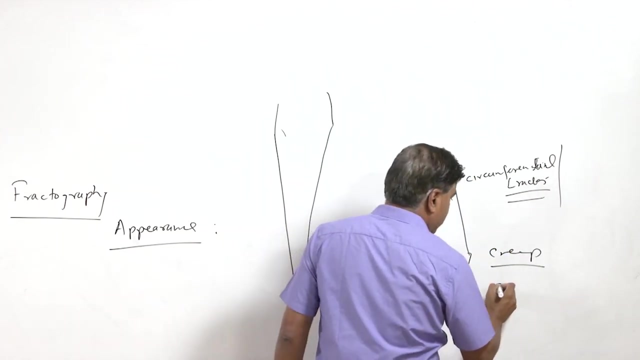 near the fracture surface there are lot of circumferential cracks. So circumferential cracks is one of the typical circumferential cracks on the component subjected to the elevated temperature and that has led to the creep. So in both the cases basically it is termed as the stress rupture because the fracture occurring at a high temperature is defined as a stress rupture, which can be of the two type where reduction in cross section takes place to such an extent that it is not able to take the external load. that will be this case, and in this case particularly where grain. 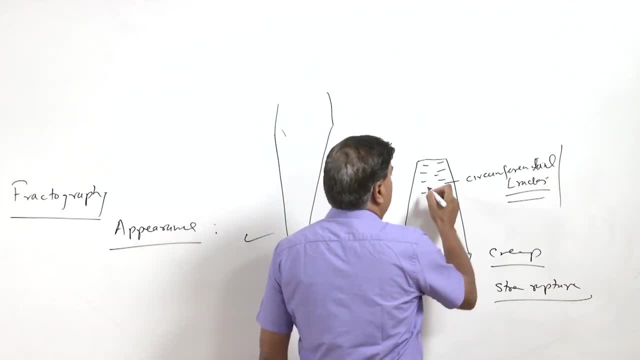 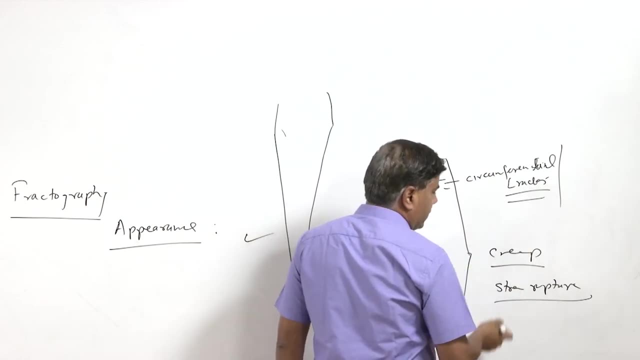 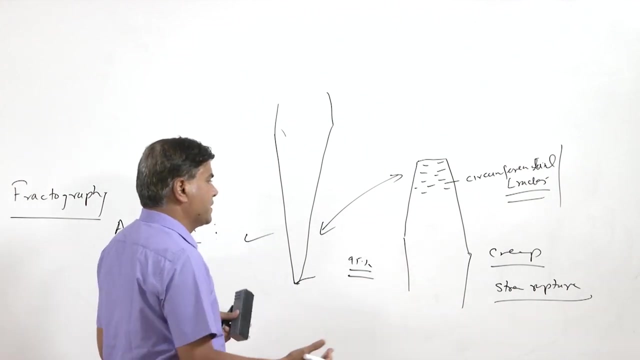 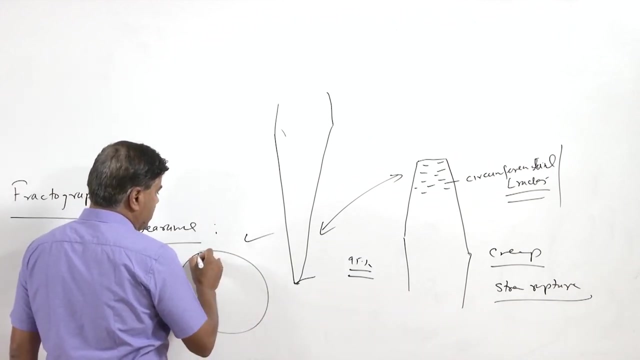 boundary sliding is so huge that lot of the circumferential cracks are developed near the fracture surface and which eventually causes the fracture. So these are the two types of the appearances of the fracture surfaces of the component which are subjected to the creep. Similarly, as I said, under the fatigue conditions, somewhere crack will nucleate and then it. 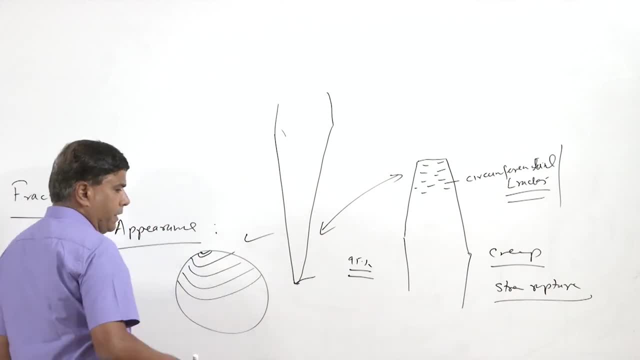 will grow like these beach marks which are. these are basically the concentric circles having the radius t- Вам fantastic- at the crack nucleation point and thereafter the sudden fracture zone. So such kind of the general features are observed in case of the footing fractures. 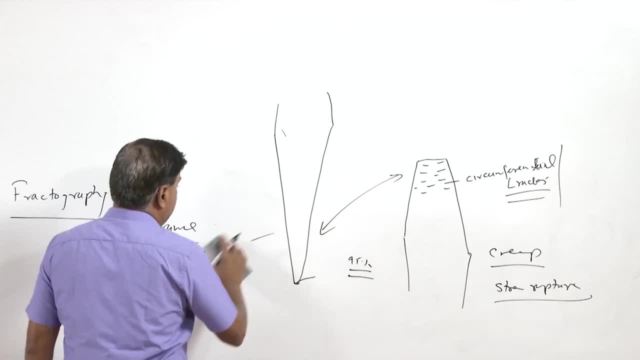 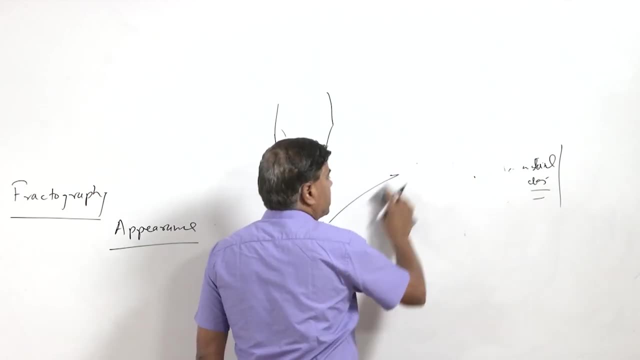 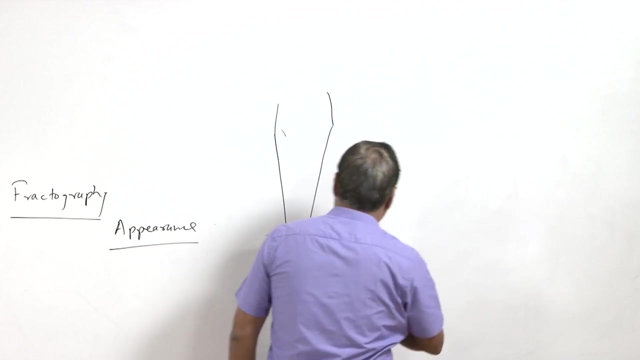 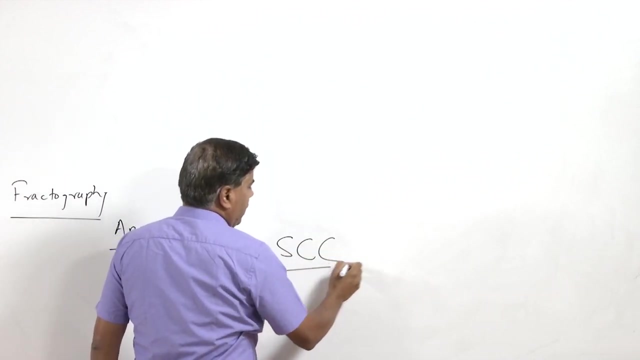 and thereafter we have one more type of the fracture, which we can say as a environmentally assisted fractures, wherein if the component is subjected to the external loading in the corrosive environment, then it will be leading to the corrosion assisted fractures, so which may be in form of, like say, stress corrosion cracking, or stress corrosion fatigue. 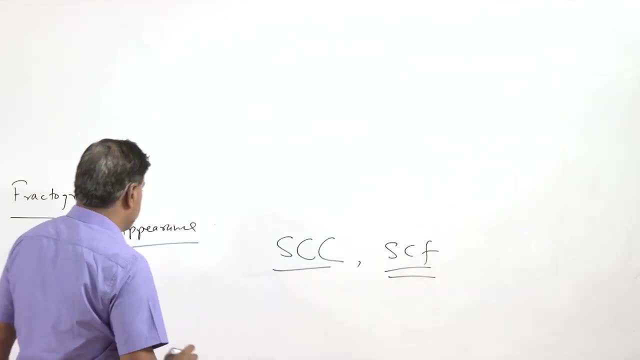 So these are the two types of the fractures where in one case, like the component is subjected to the external tensile stresses and in corrosive environment, some cracks nucleate and they grow in very localized manner, So like in branched manner, and then the crack will be growing gradually and eventually fracture. 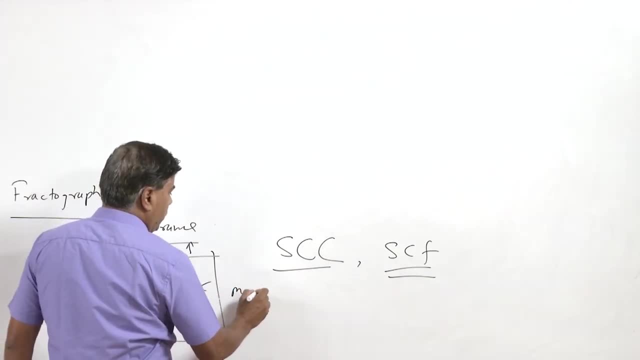 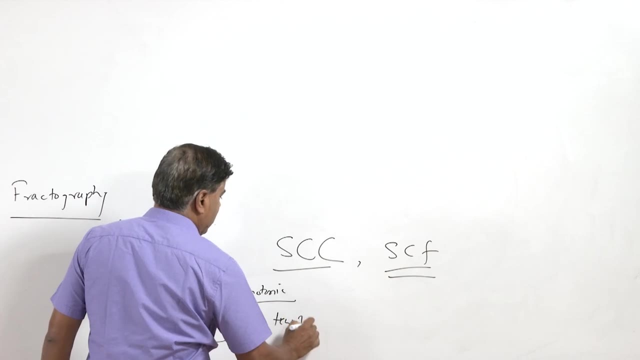 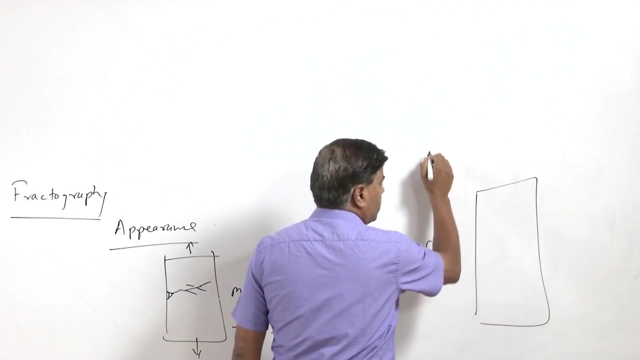 will be taking place. So in this case the load is monotonic. in case of the stress, corrosion, cracking, of course it has to be tensile and on the other hand, when the component is subjected to the exposed to the corrosive environment, so corrosion will be causing the pits and the crevices. 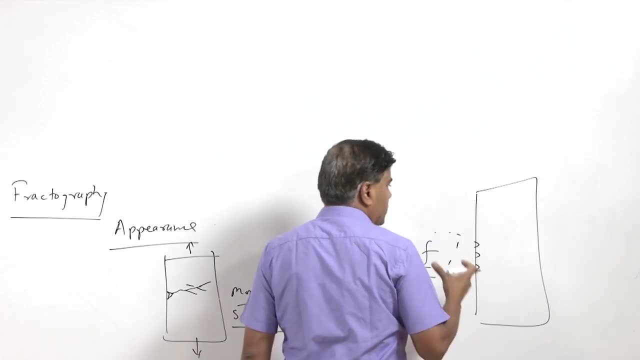 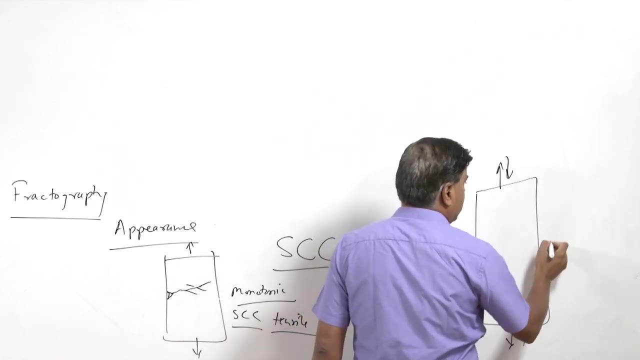 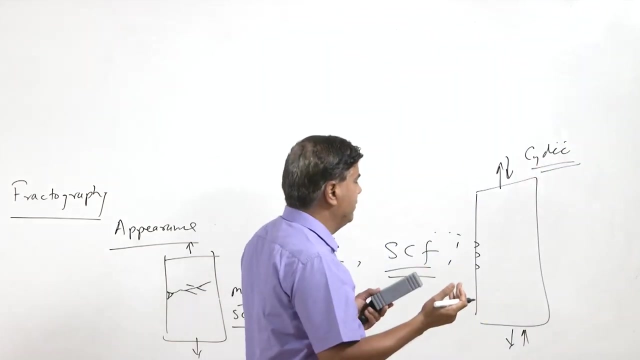 here and there. So as per the corrosion sensitive zones, and if it is also subjected to the fluctuating loads, so in that case, so you can say, component subjected to the cyclic loading, at the same time it is also exposed to the environmental, corrosive environment. then out of these number, 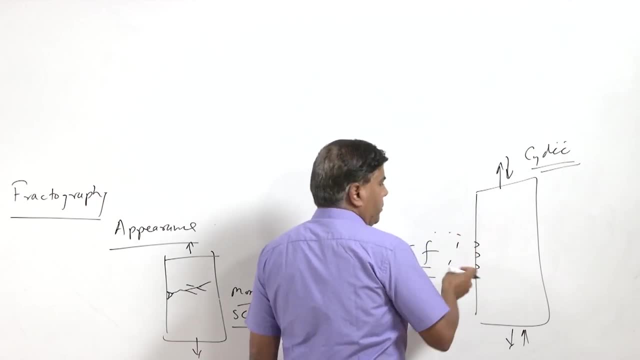 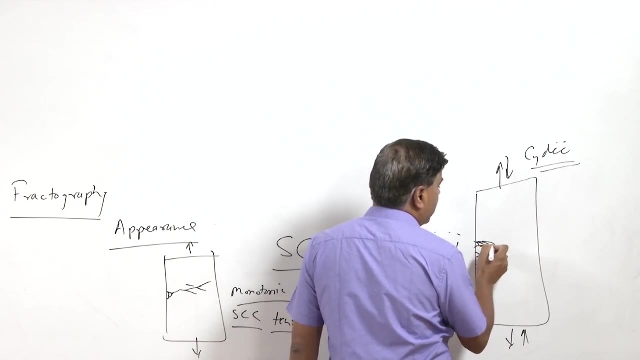 of the pits and the cavities which are which have developed at the surface due to the corrosion. some of them will grow And then under the fatigue conditions, So this is the case. So cyclic loading conditions and their growth eventually will cause the fatigue fracture. So here such kind of fractures are very fast and in this case the nucleation is facilitated by the pits and the crevices which are being generated at the surface, and the cyclic loading will be facilitating the growth of crack and eventually the sudden fracture will be taking. 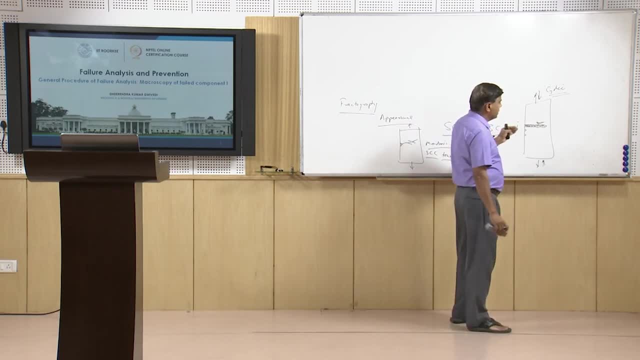 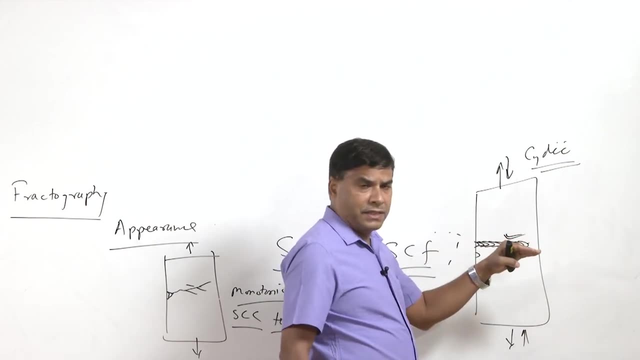 place as soon as the cross section is reduced to some extent. So this is the case. So the friction is reduced to such an extent that the external loading is beyond the capacity of the load resisting cross sectional area left out, and then sudden fracture will be. 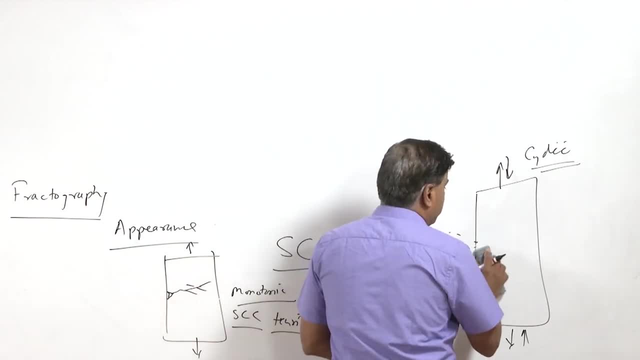 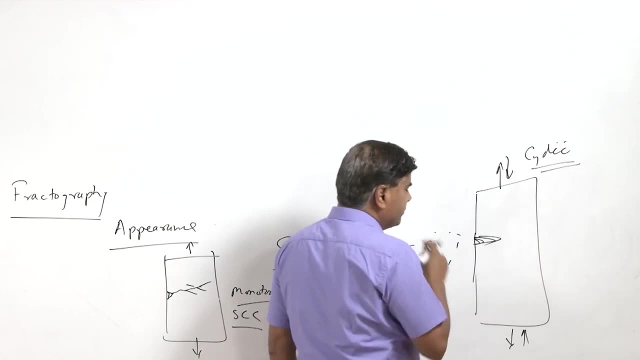 occurring. So that will depend upon the fracture toughness of the material, like if the low fracture toughness material, the crack will be growing up to such an extent and then thereafter sudden fracture will be taking place. but in high fracture toughness material the crack can grow gradually. 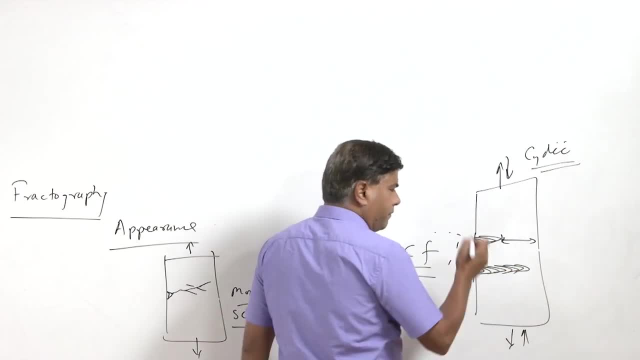 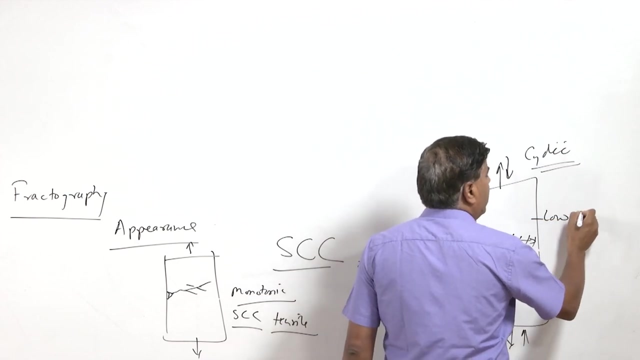 and thereafter the sudden fracture will be occurring when the left load resisting cross sectional area is reduced to a great extent. So in this case load resisting cross sectional area is large in case of the low fracture tough materials, and this is the case of the high fracture tough materials, So, depending upon the fracture toughness of the material, The third stage of the fracture toughness of the material is the fracture toughness of the material. So the third stage of the catastrophic fracture will vary and that will decide the extent up to which the crack can grow during the cyclic loading prior to the catastrophic fracture. 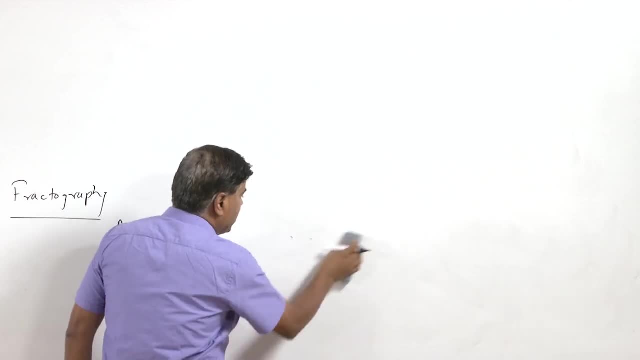 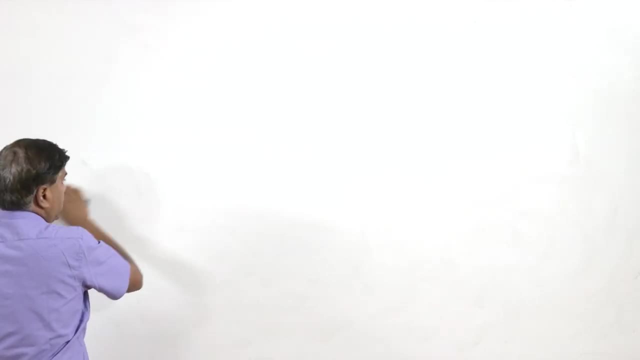 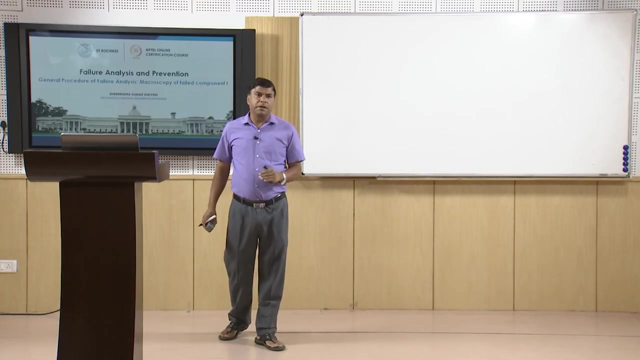 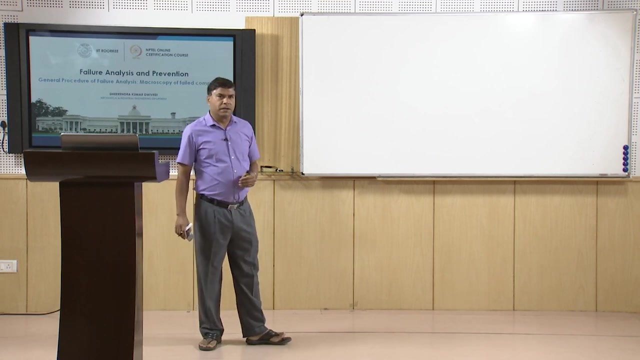 So these were the categorization or the types of basic types of the fractures based on the appearance. So, based on the appearance, we have ductile fracture, Brittle fracture, fatigue fracture, creep and environmentally assisted fractures like stress, corrosion, cracking and the hydrogen embrittlement. 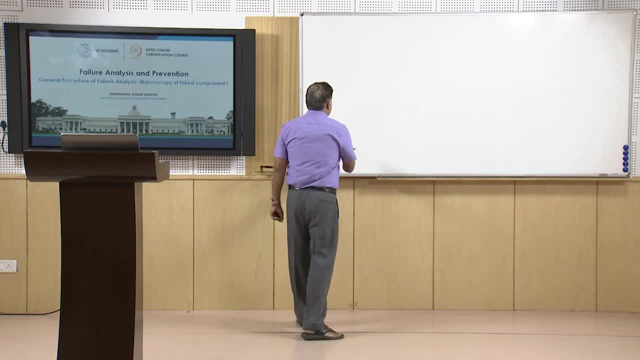 So now, if you have to make the useful observations and inferences after observing the failed component, say visual examination, or the macroscopic observations, Then all the possible observations will be made Then, or the microscopic observations, then what observations we can make in with regard? 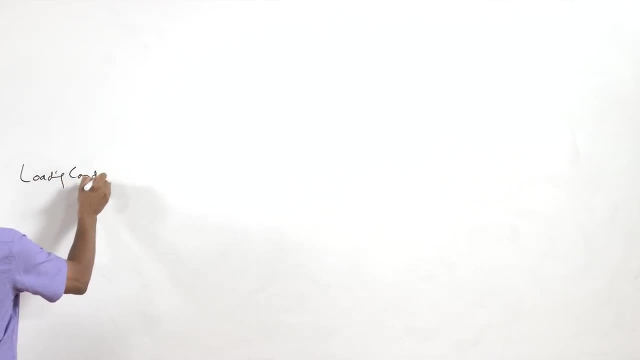 to the loading conditions. So, with regard to the loading conditions, loading can be like, say, like static, or we can say the monotonic or cyclic where load is varying or changing or fluctuating. so cyclic loading, So in case of the monotonic loading, and in case of the cyclic loading, so in case of 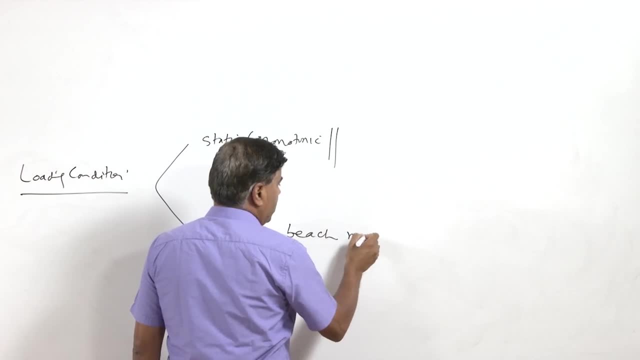 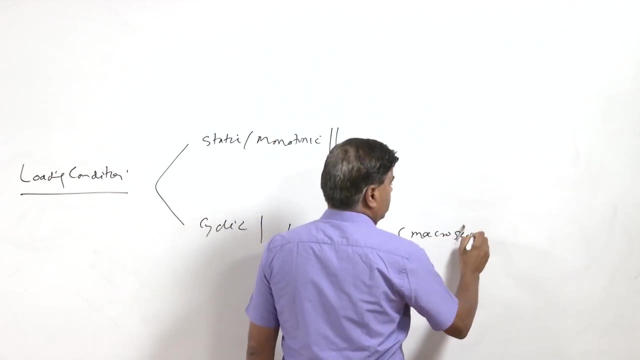 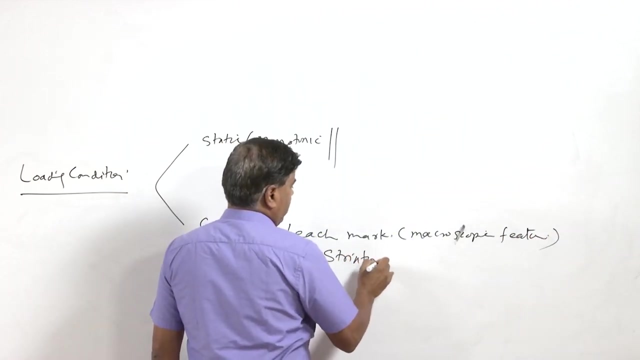 cyclic loading. we can see the beach marks, which is a macroscopic feature, or we get the striations on the fracture surface striations, which is a microscopic features. we do not get the striations, So we do not get the macroscopic features. 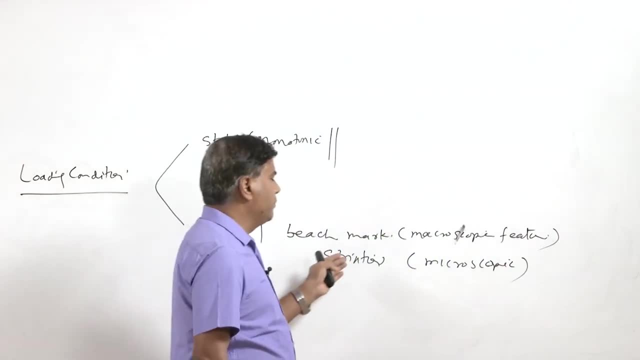 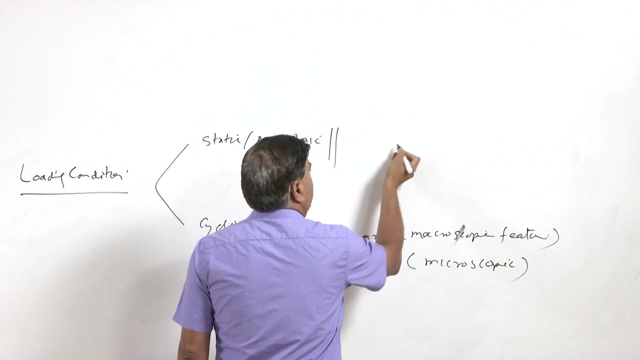 The naked eye. low magnification lenses, so the we need the scanning electron microscope to observe these striations. On the other hand, no such kind of the beach marks or striations will be there on the fracture surface, So they will be the static or the they will be the monotonic fracture. so for this case, 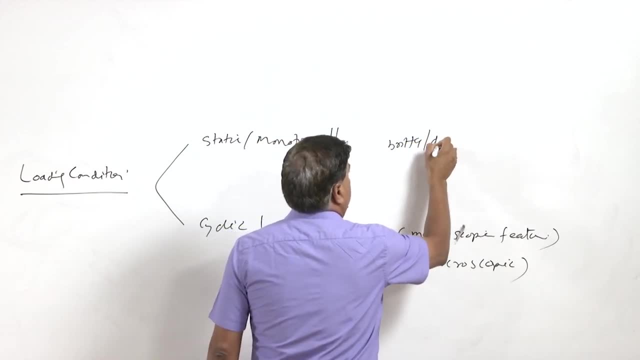 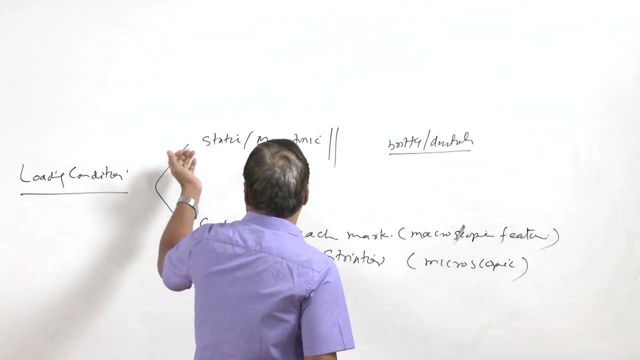 we have, like the brittle or the ductile fractures of which like say, this is the case of the, in case of the monotonic loading. So there is no special feature like beach marks or striations in case of the static and the monotonic loading. 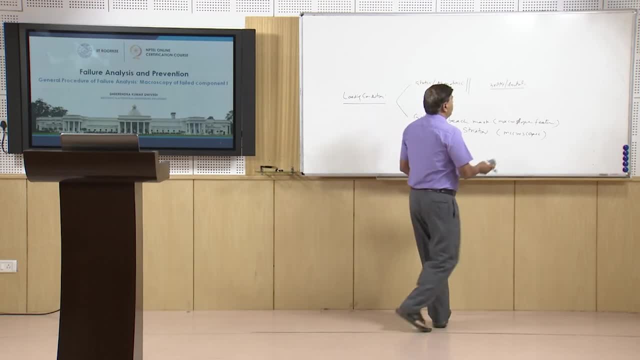 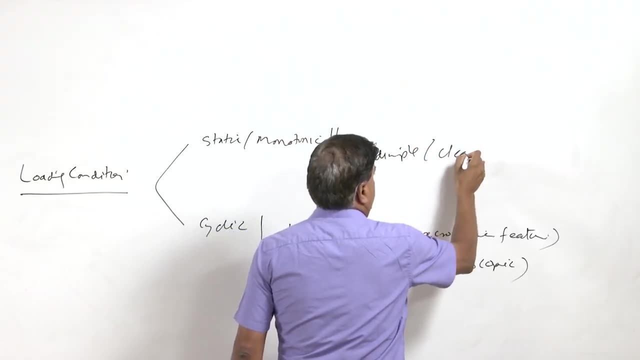 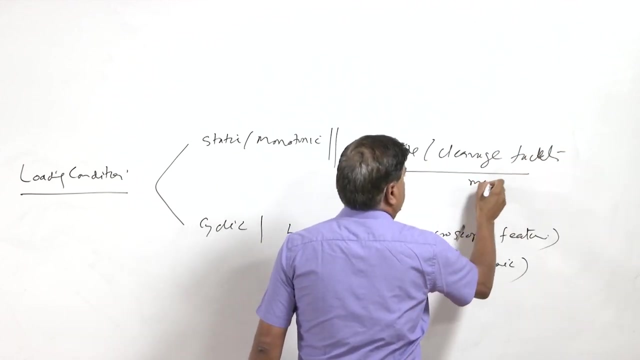 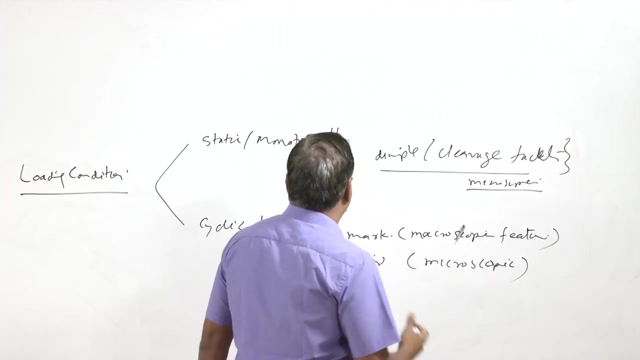 There are other microscopic features which are used to define if the fracture has occurred, either like dimple or the cleavage facets. their presence will. so these are the microscopic features which will indicate that the loading has been the monotonic and which will be leading to 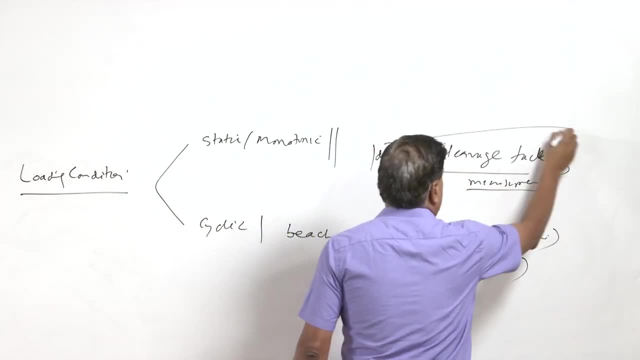 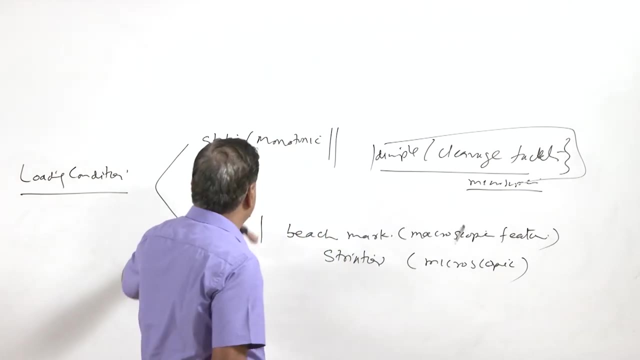 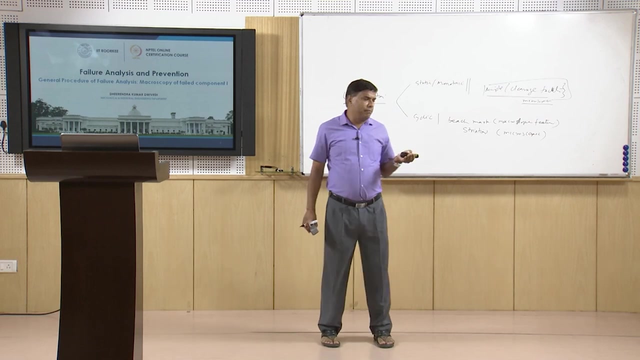 the either ductile or the brittle fracture, But these features are different than what we get in on the fracture surface in form of the beach marks or striations for the cyclic load, and there is no special feature as such which can be observed using the naked eye or macroscopic observations. 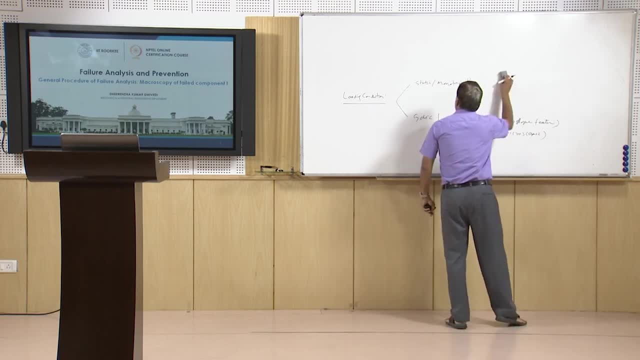 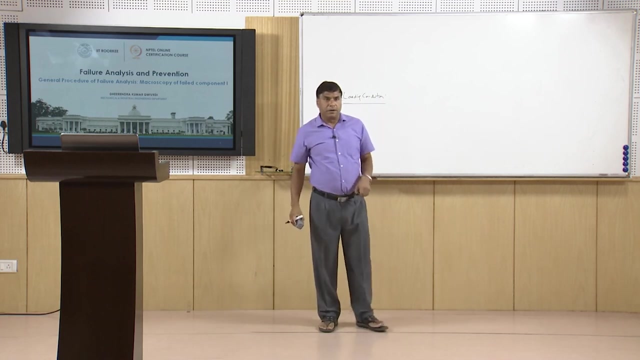 Macroscopic observations to say that this is the monotonic loading, so be indication of the beach marks will suggest the cyclic loading, and absence of any such kind of the feature will indicate the possibility of the static load. Then the macro scale. based on the macro scale observations, the fracture is a ductile or it is brittle. so in this case, in case of brittle, there is no major change in cross section area of the fractured component like this. So the component, Whatever cross section is here, same is near the fracture surface, while major change in cross section area is observed in case of the ductile fractures. 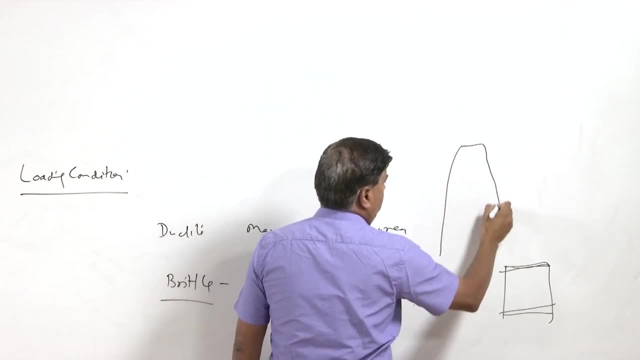 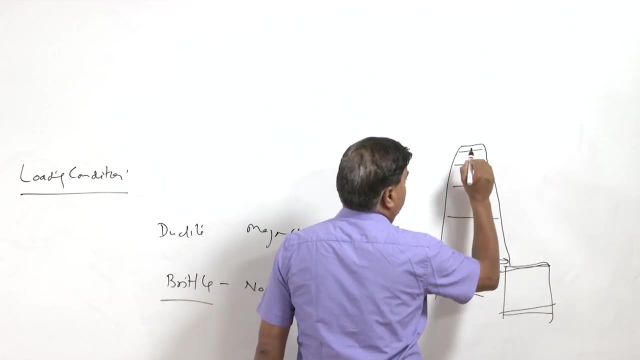 So this may be in this form, where there has been lot of change, in that this is the initial diameter and there has been reduction in the diameter and near the fracture surface the significant reduction in the diameter has taken place. So we are saying that this is the ductile fracture. 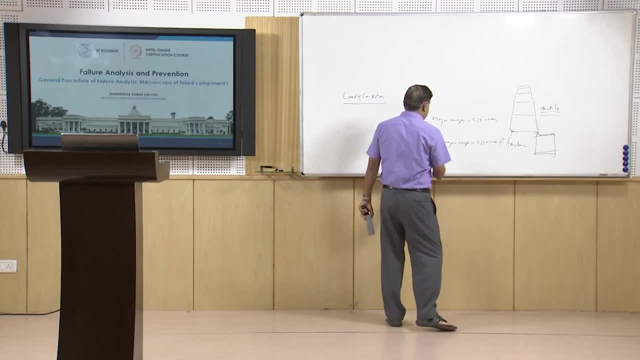 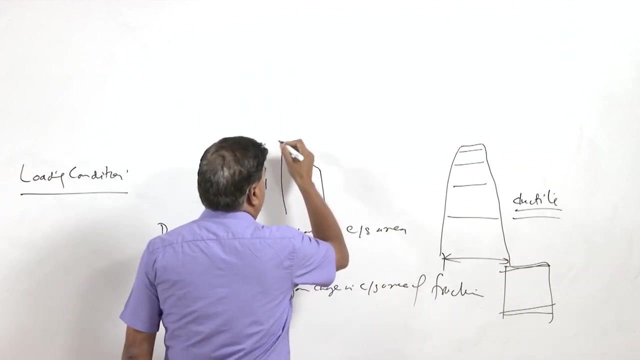 And at the same time, like in case of the ductile fracture, it is feature. in the case of the ductile fractures it may be like the with the shear lift fracture. the surface fracture surface may have the shear lifts or the slant fracture surface. Slant fracture. 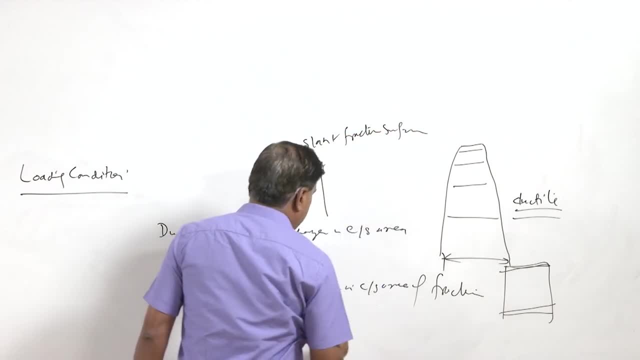 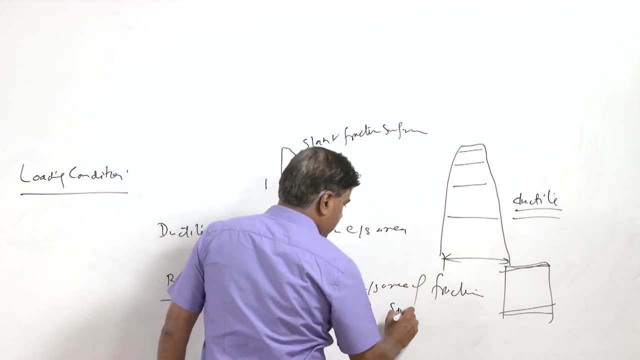 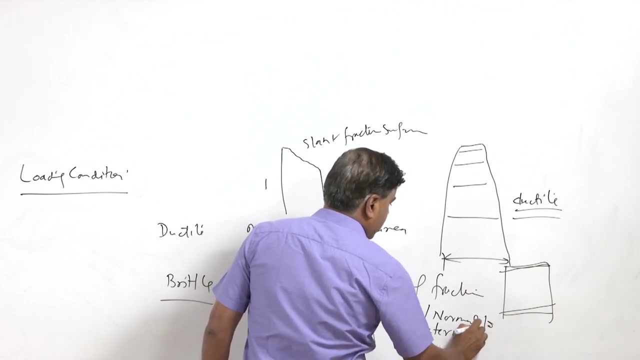 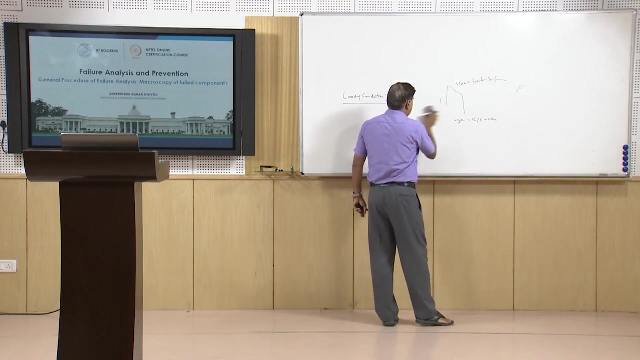 Slant fracture, Slant fracture surface, and it may be the fracture surface is normal to the external loading. So the square, or you can say the fracture surface is normal to the external loading. Then, third one is like the macroscopic observation with regard to the mode of the fractures.